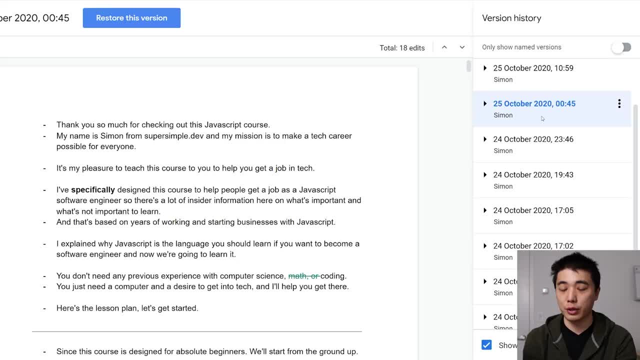 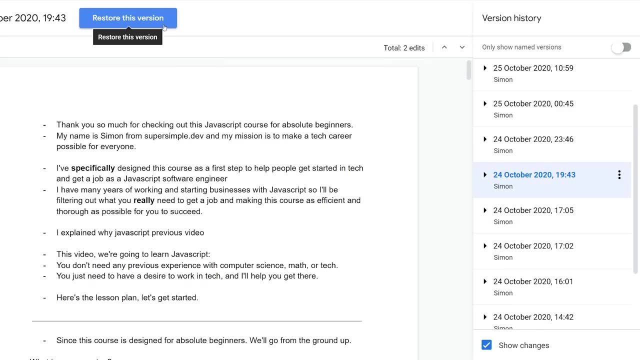 document in a version history like this, And this makes it easy for you to go back to previous versions of your document or to restore your document back to a previous version in case you mess up. Git is basically the same thing. It's a version history for our code, So it allows us to. 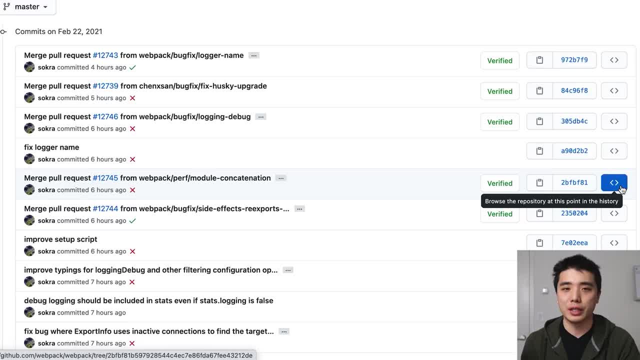 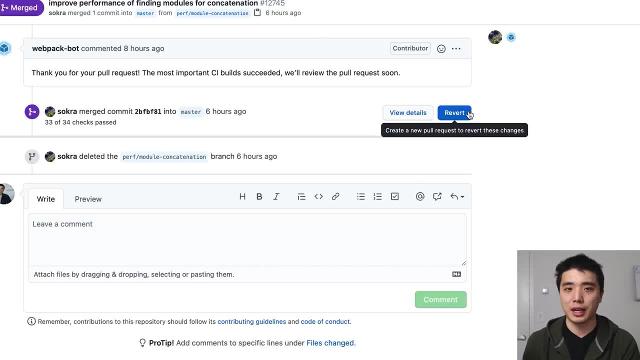 save past versions of every file of our code and then, whenever we need to, we can view the code that we had in the past, or we can restore all of our code back to a past version. It's basically a safety net when we're developing software, But that's just the tip of the iceberg. 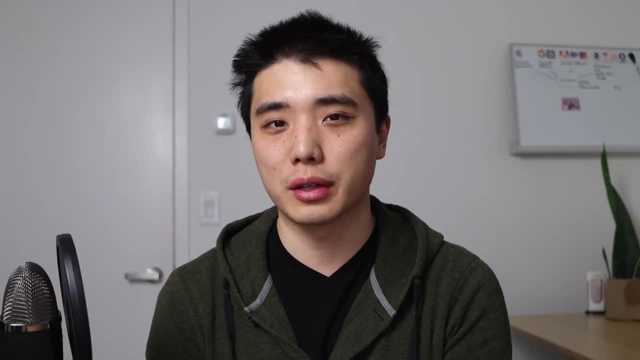 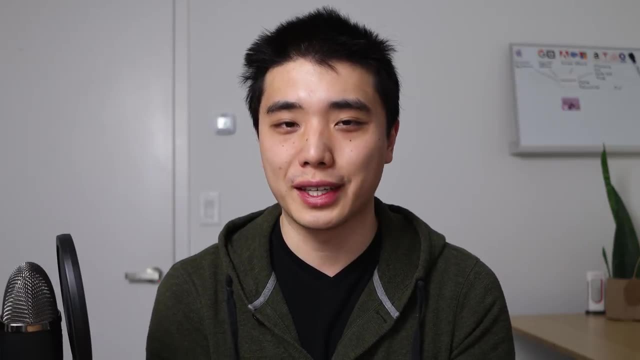 Version history is just a small part of what Git can do, And later on we're going to learn additional skills like GitHub and branching. that's going to take you to that professional level. But for now, we're going to start off by learning how to use Git to recreate the Google Docs version. 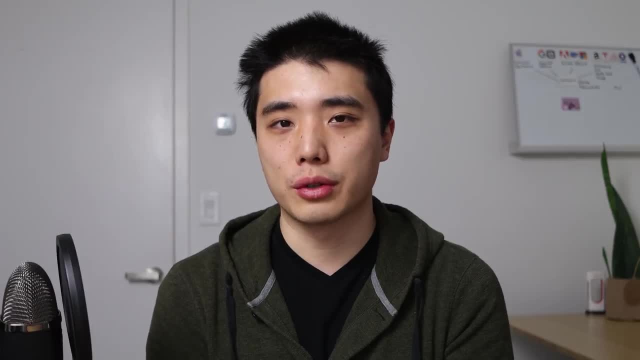 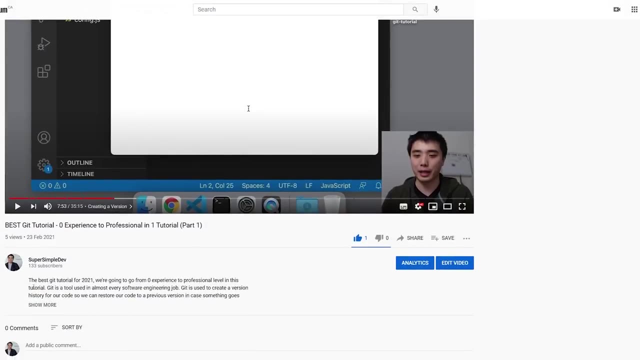 history feature. for our code To follow along with this tutorial, you just need to have written some code before. You don't need any prior experience. I'm going to explain every step that we do. You can find the different sections of this tutorial in the description. 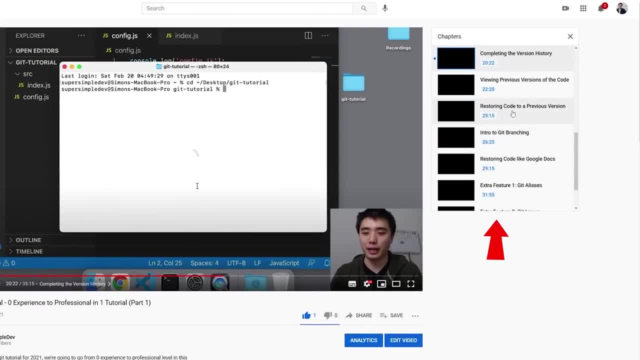 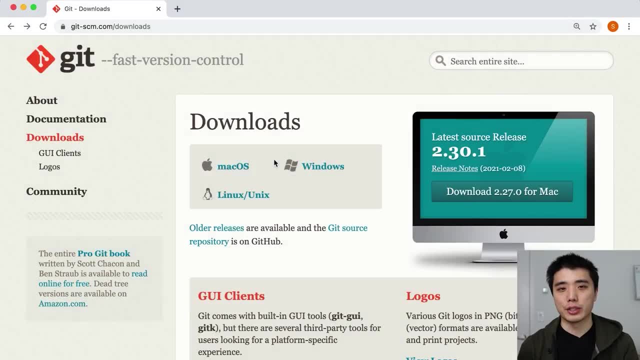 in the timeline or by clicking here. With that said, let's get started with the tutorial. First, let's learn how to install Git. If you already have Git installed, you can skip to this time in the video. The installation process is pretty simple. 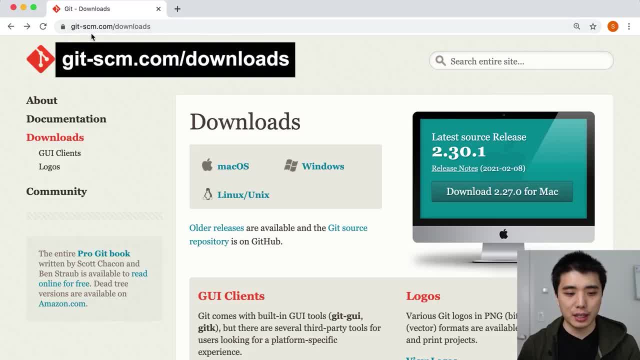 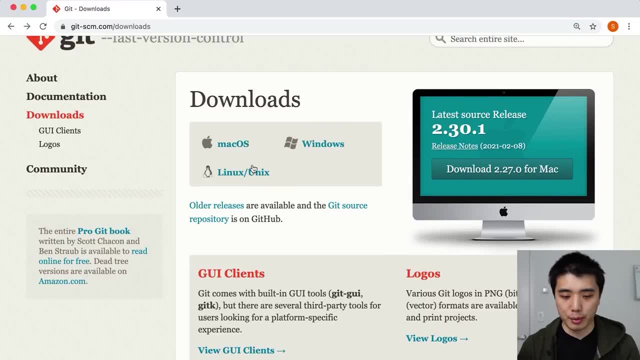 You just have to go to this website, git-scmcom downloads. I'll leave a link to that in the description, And then what you're going to do is to pick the operating system that you have. I'm going to start with macOS. first, Windows users. 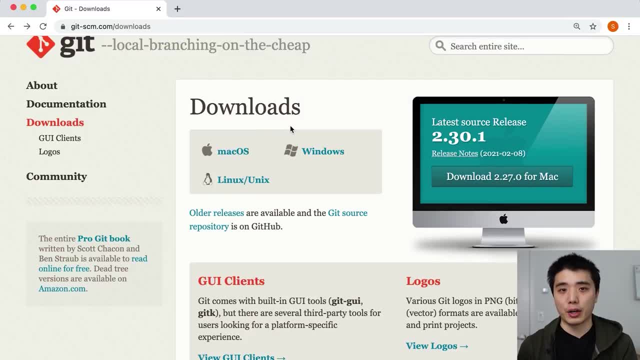 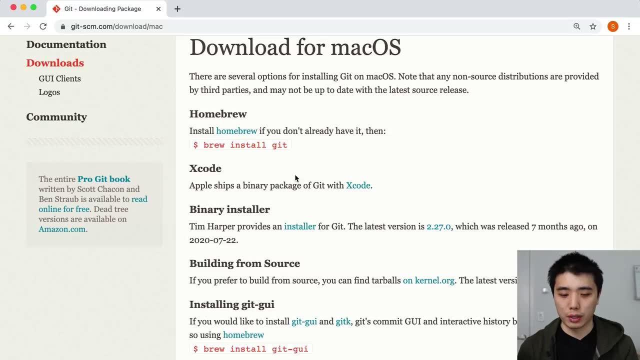 you can skip to that And then you're going to pick the operating system that you have. I'm going to necessarily go to the browser I just showed you For macOS users. we're going to go into this section. You'll see we have several options here. The recommended option for 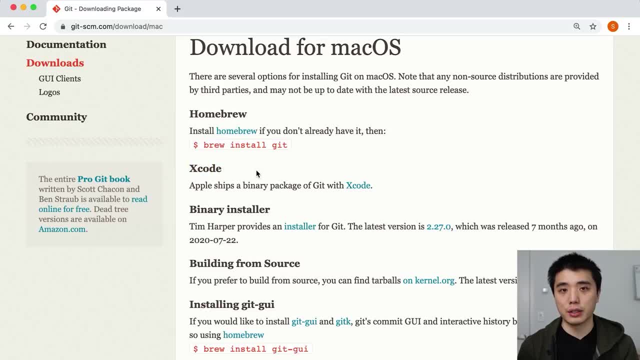 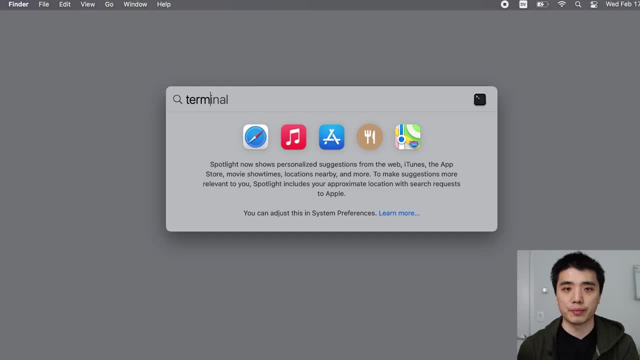 installing Git is to install excode There. two ways to do that. The first way is to click on this icon, which will open Spotlight. Then we're going to search for terminal and we're going to open Terminal. If you find that the font is too small, you can go. here and then click on terminal, Then you can open thechiedonline, then tap here, Then you can go restock, do it here and you can update the file. as you go onto promo region of your computer and tool page, Just pick what is want for the capabilities and inside of this video is here Once you have the kit. 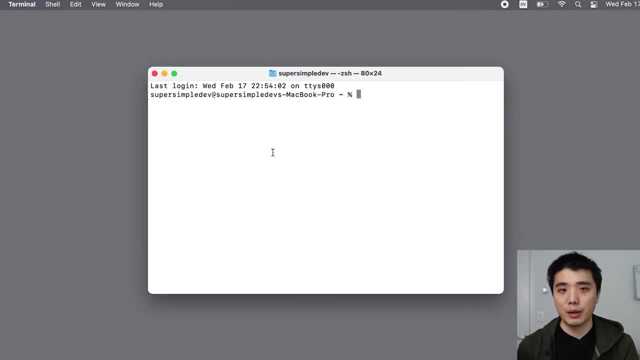 here to change the font size. So now that we have terminal open, we're going to type in git and then we're going to press enter. So if you see a message like this, that means that git has already been installed and you can skip to this. 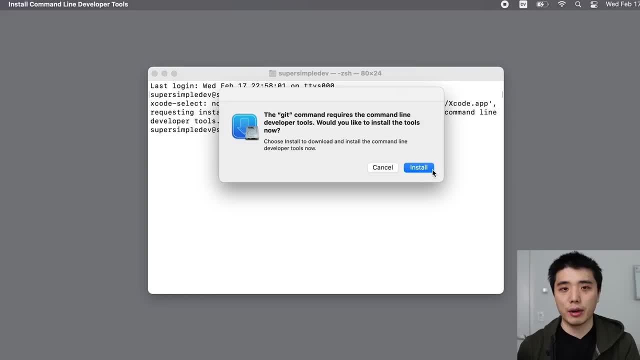 time in the video. If you see a pop-up like this, go ahead and press install and that will install git for you. When that installation finishes, we're going to close the terminal and we're going to reopen it, and then we're going to type. 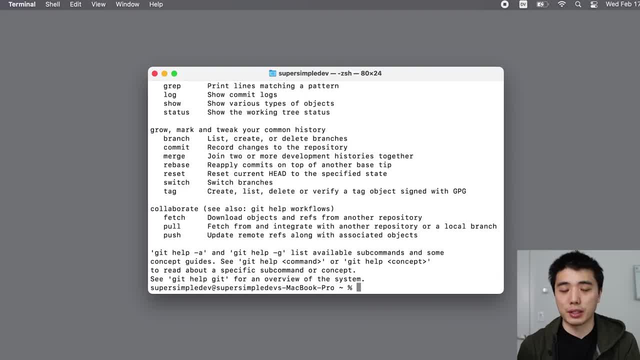 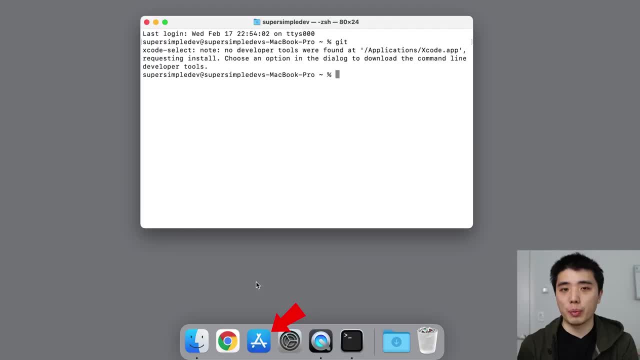 in git again and press enter, So you should see a message like this, which means that git has been installed. If that didn't work for you or the pop-up didn't show up, you can also open the App Store and then search for xcode and. 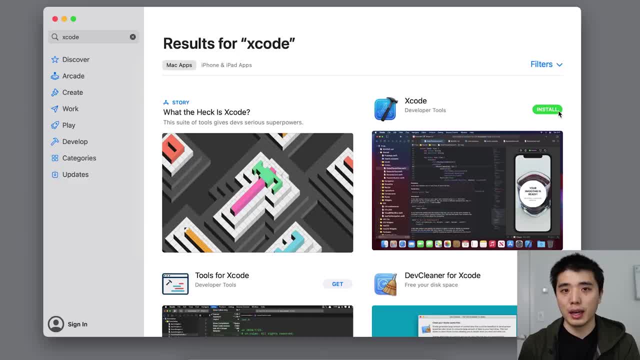 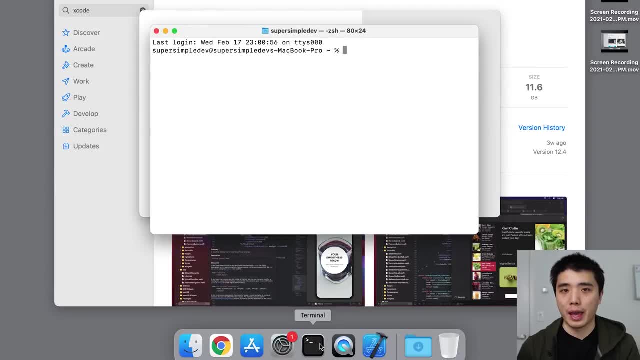 then install xcode. After xcode finishes installing, we're going to open it for the first time, and then we're going to close and restart our terminal, and then we're going to type in git and press enter again. Now, git should have been. 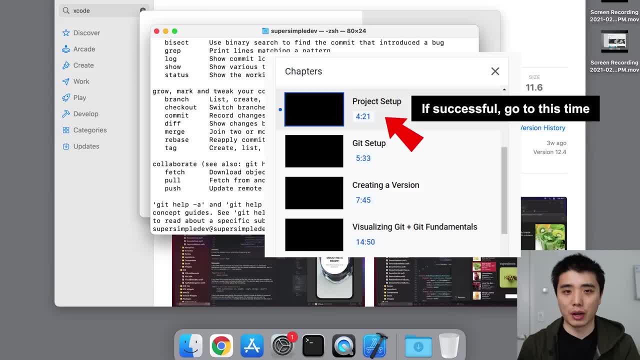 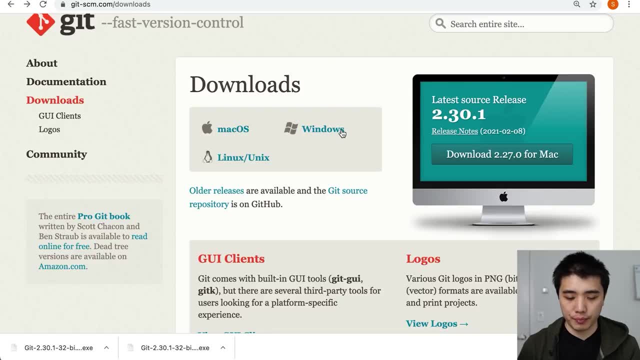 installed, and if it doesn't work, let me know in the comments and we'll figure out what's going on. For Windows, the installation is pretty simple. We just have to go to this Windows section and the installer will download automatically. If it doesn't, you can also. 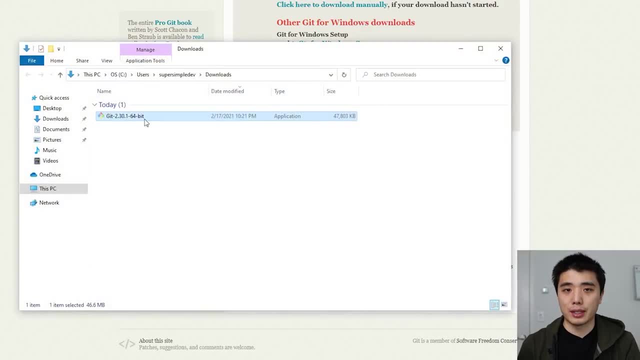 click this link After the installer finishes downloading. we're going to open it and then we're just going to run the installer So we can keep all the default options. just click next until you're finished installing. After that's done, we're going to search for a program called PowerShell. 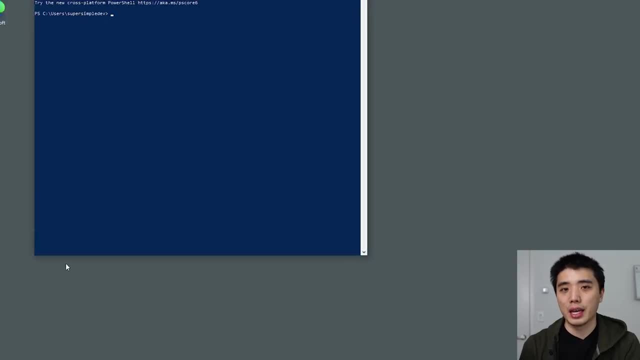 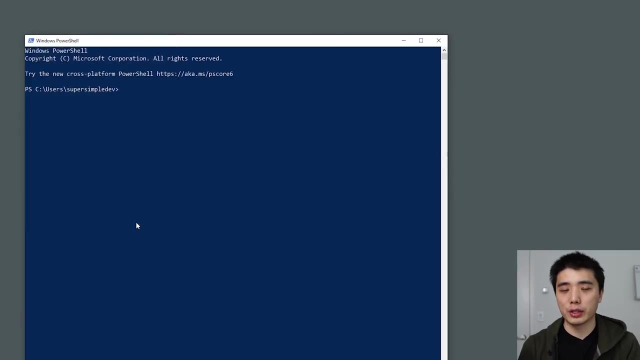 We're going to open Windows PowerShell. If you find that the font is too small, you can click here and click here to change the font. So once PowerShell is open, we're going to type in git and press enter, So you should see a message. 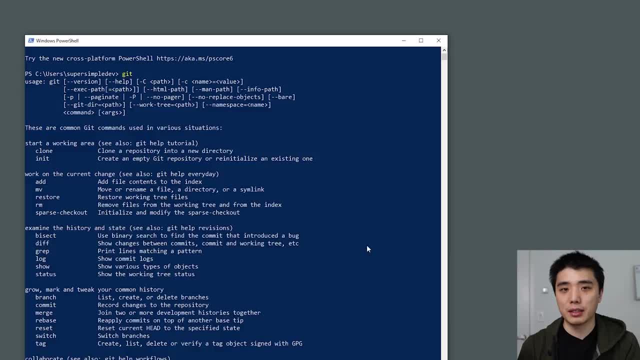 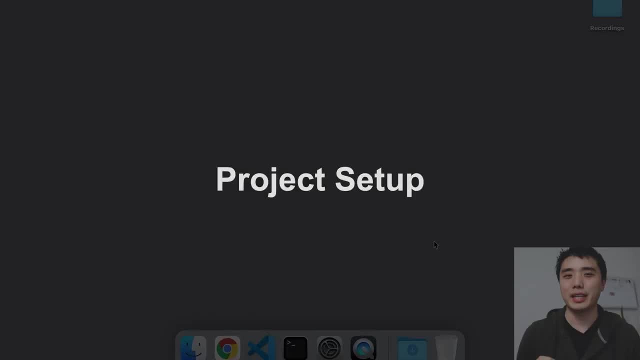 like this, which means that git has been installed. If you don't see that message, let me know in the comments and we'll try to figure out what's going on. Now that we've installed git, we're ready to learn how to use it to. 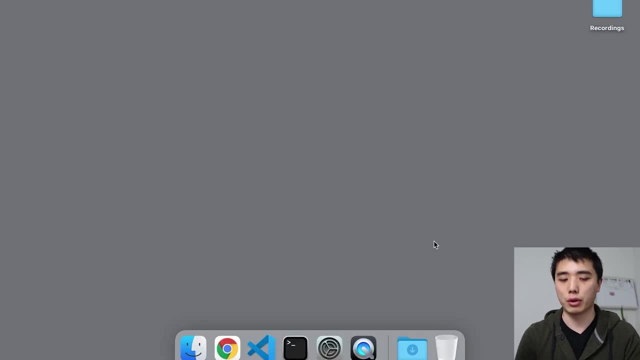 build this version history for our code. So I'm going to be doing this tutorial on a Mac, but the steps are the same whether you're using a Mac or a Windows computer. So the first step that we need to do is to have some code to practice. 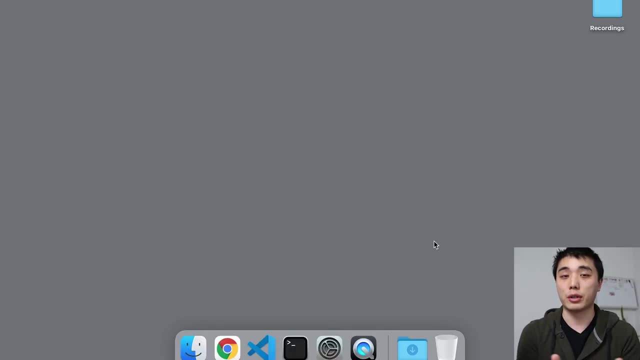 with. So if you have your own code or your own project that you want to use, feel free to use that. Otherwise, we're going to create some code quickly right now. So I'm going to go to my desktop and create a new folder that's going to: 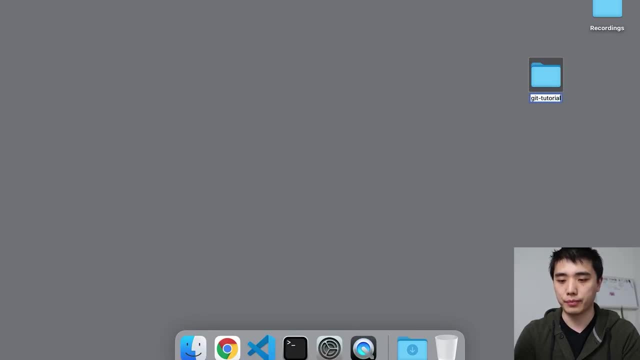 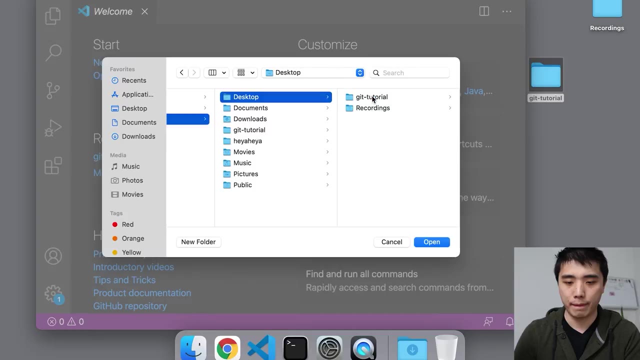 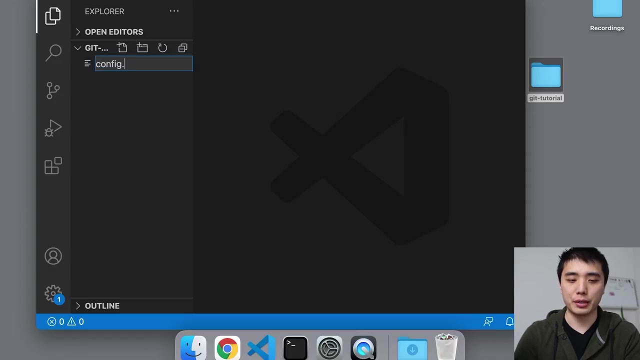 contain all of our code. I'm going to call it git tutorial and then I'm going to open this folder in my code editor. So I'm just going to type out some example code that we can practice with. If you want to copy this code, feel free to pause the video if you need to. 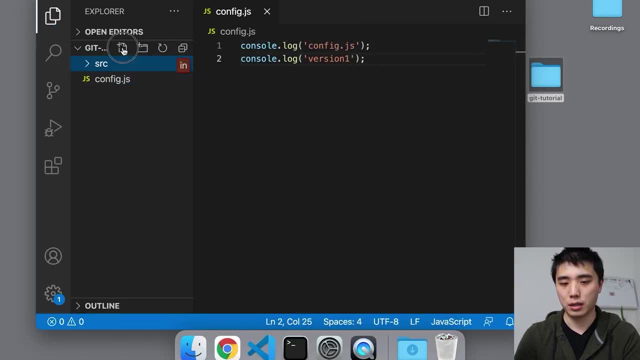 Okay, so this is our example code. We just have a console log statement with a file name and then a console log with version one, just so that we can track which version that we're on, since we are building a version history. It's pretty simple. 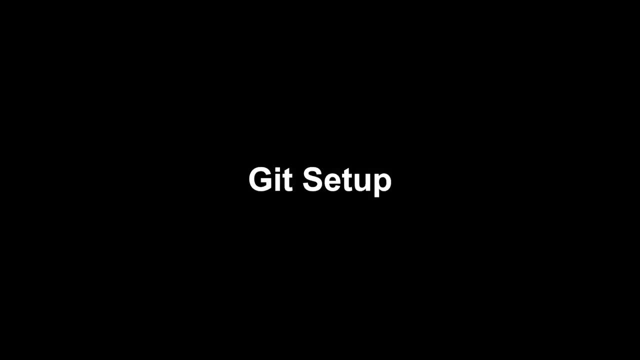 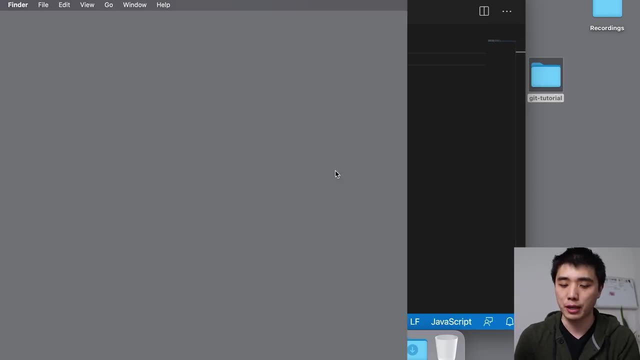 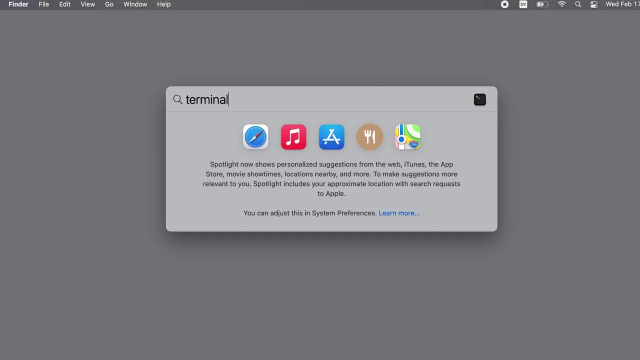 we just need something to practice with. So git is mainly used from the command line which is terminal on Mac, or PowerShell on Windows. To open the command line on a Mac, we're gonna click this icon which will open Spotlight, and then we're gonna search for terminal. 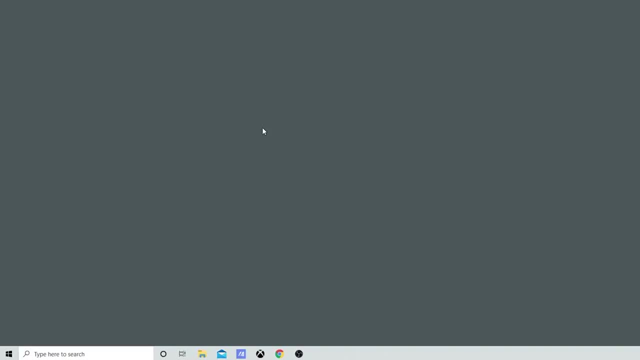 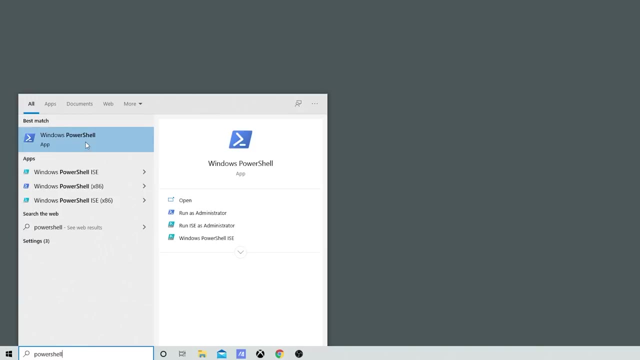 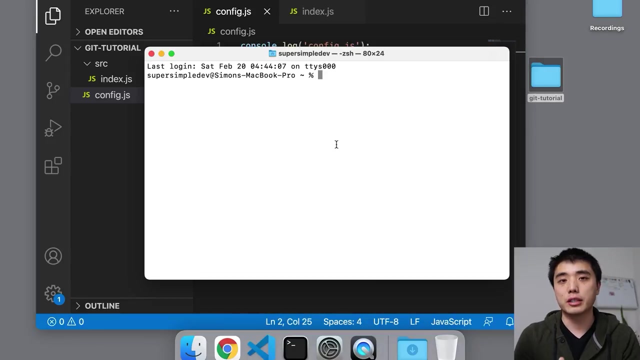 and then we're gonna open terminal To open the command line on Windows. we're gonna search in the start menu for the program PowerShell and then we're gonna open Windows PowerShell. So let's go ahead and open that up. So you don't need to know a lot about the command line. 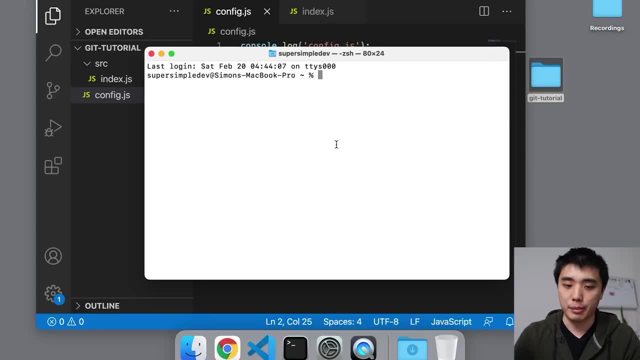 to use git. but you do need to understand one concept: The command line is where we can give commands or instructions for the computer to follow. So, for example, I can give this command ls, and when I press enter, the computer will follow this command. 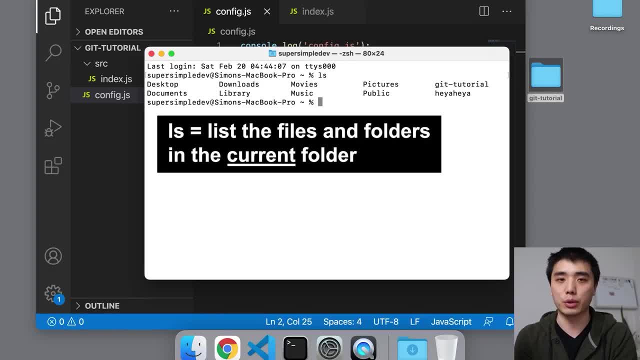 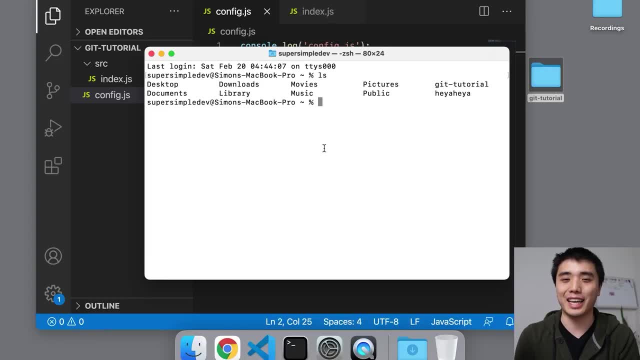 and list the files and folders that are in the current folder. So notice that I said current folder. So the concept you have to understand is that all of the commands run inside a specific folder. So when we first open up the command line, the commands are running inside a special folder. 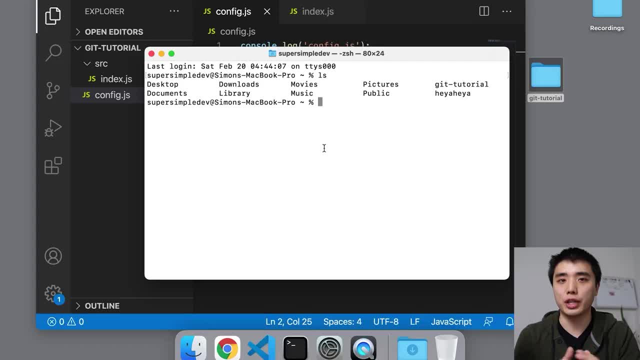 called the home folder. So in order to use git, we need to change the folder that the commands are running inside of to this folder which contains all of our code. So to do that, we can give this command cd, which stands for change. 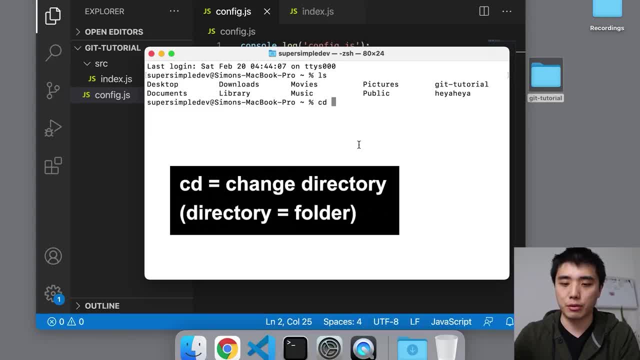 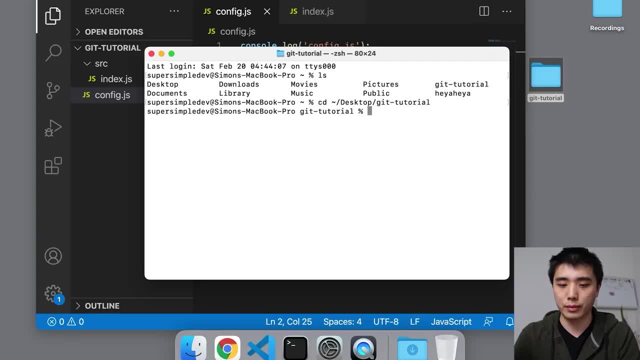 directory. directory is the same thing as a folder and we're gonna change the directory to tilde slash, desktop slash, git tutorial. And let's verify that we're in the right place by giving the ls command again to list the files and folders. 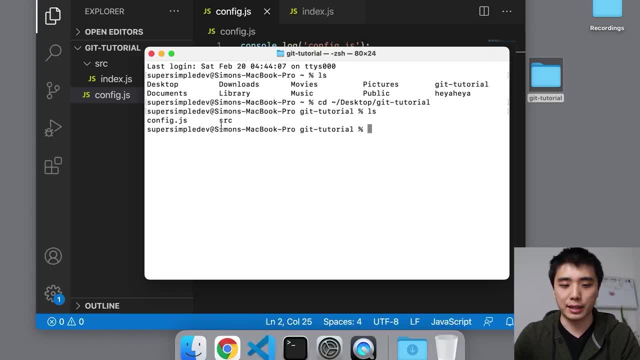 that are in the current folder. So, as you can see, we have configjs and source here which matches what we have in our code editor. so we know we're in the right place. So one last thing you have to know about the command line. 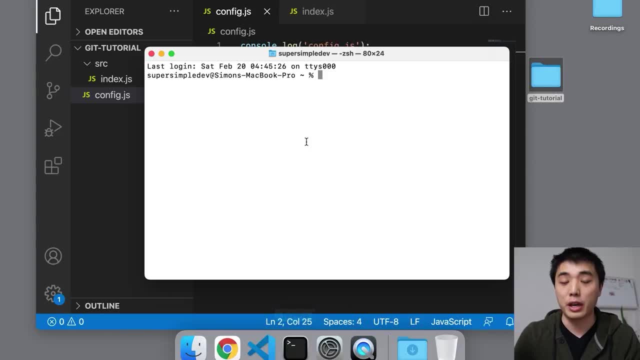 is that if you ever close the command line and then you restart it, you're gonna start inside the home folder again. So make sure that the first step you do is to change directory back into this folder which contains all our code, And that's it. 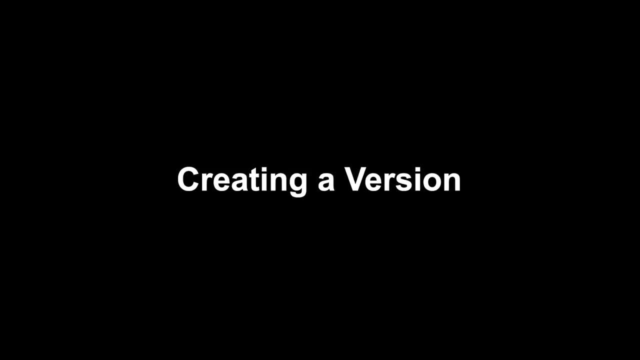 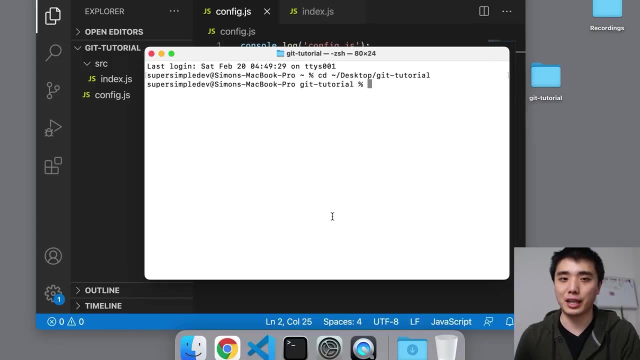 Now we're ready to learn some git. Now let's create the first version of our code in the version history. So the first thing we need to do is to set up git inside this folder that contains our code, And to do that, we're gonna give this command. 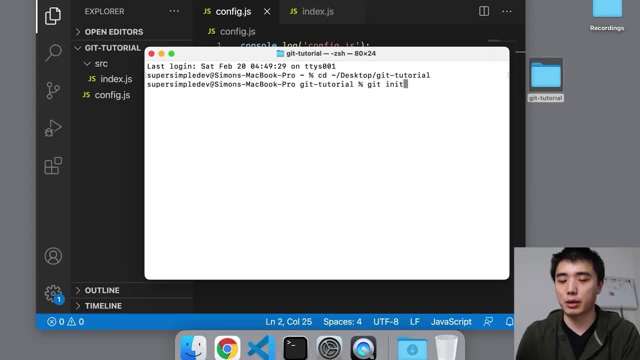 git init And to run the command we're gonna press enter. So what this does is that it sets up git inside this folder and git is now tracking all of the files in this folder for changes And don't worry about memorizing these commands. 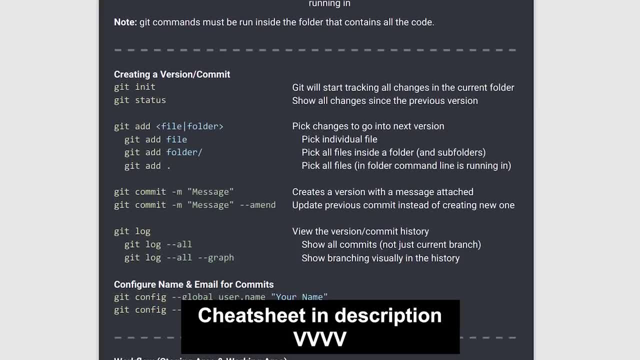 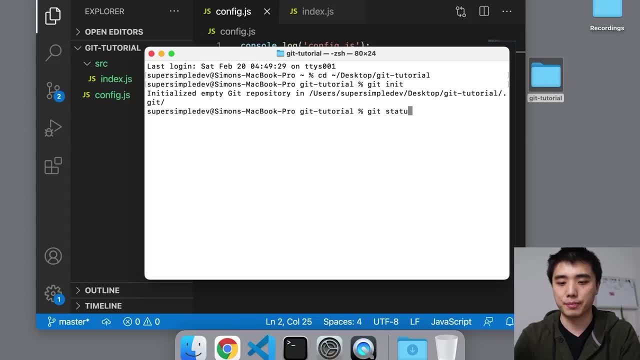 because I'm gonna put all the commands that I teach you in a cheat sheet that you can find in the description below. So the next step we're gonna do is we're gonna run another command called git status, And what this does is that it tells us: 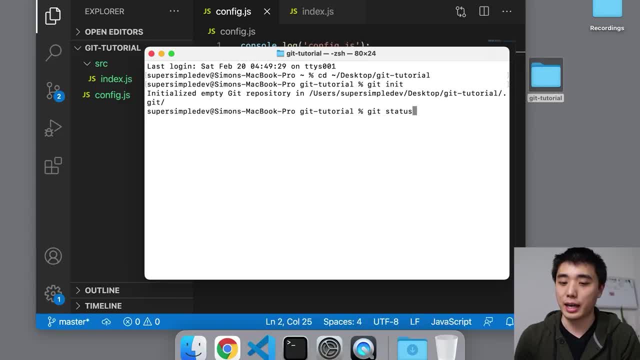 what changes have been made since our previous version. And since we don't have a version right now, we're just gonna see that we have some new files, So let's go ahead and run this command. So there's a lot of text that comes out. 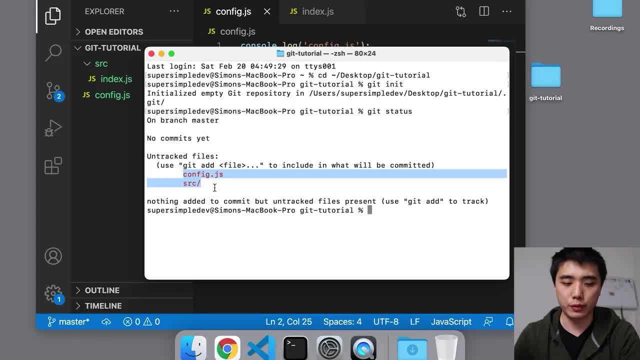 The most important part is here. So git is just telling us that there is a new file called configjs and a new folder called source that are not being tracked in our version history, And that is correct, because we actually don't have a version history. 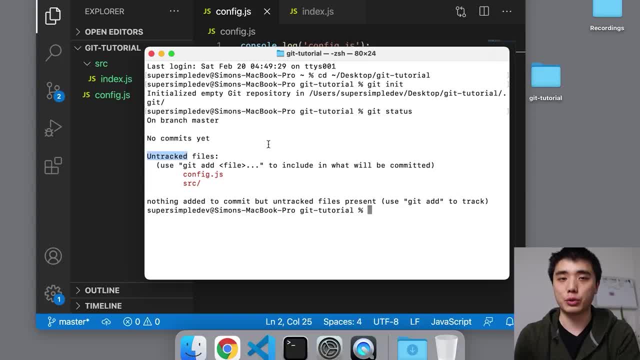 So our next step is to create our first version, And we have to do two things to make this happen. The first thing we have to do is to pick a file, pick which changes we want in our next version, And to do that we're gonna use this command: git add. 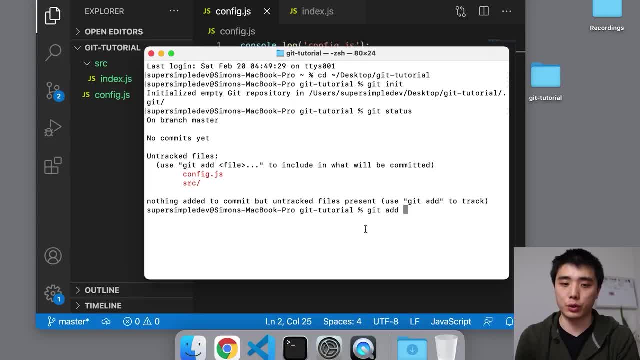 So git actually allows us to pick which changes we want in our next version. So we actually don't have to have both of these in the next version. We can actually just pick configjs by adding it like this. So if we give this command, 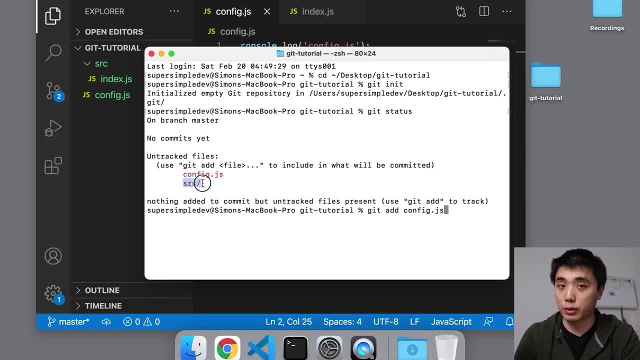 git will only put this in the next version and this source folder will be left out. On the other hand, if I give a folder to git add, it's going to add all of the files inside the folder, including any subfolders. So for our first example, 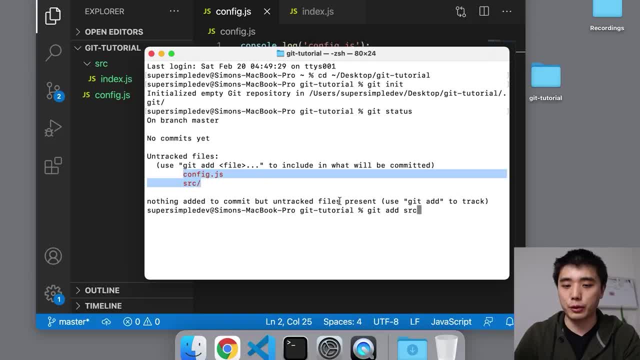 let's just add both of these into the next version, And a shortcut for doing this is git add dot. So the dot in command line represents the current folder that the command line is running in. And if you remember at the beginning, when we started up the command line, 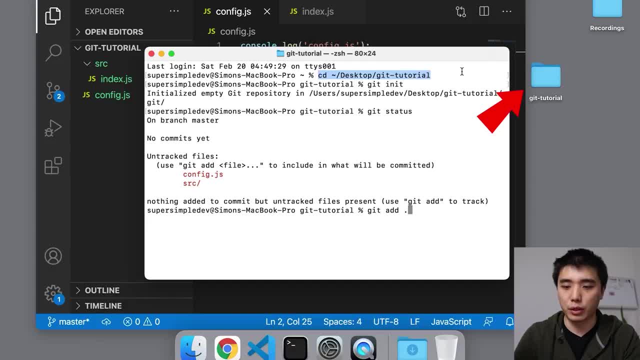 we changed the folder that the command line is running in to this folder, which is this folder that contains all of our code. So if I say dot here, we're gonna add everything in here, including any subfolders. So that's a good shortcut you can use. 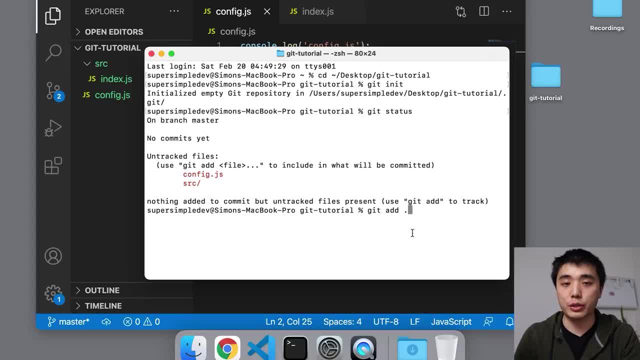 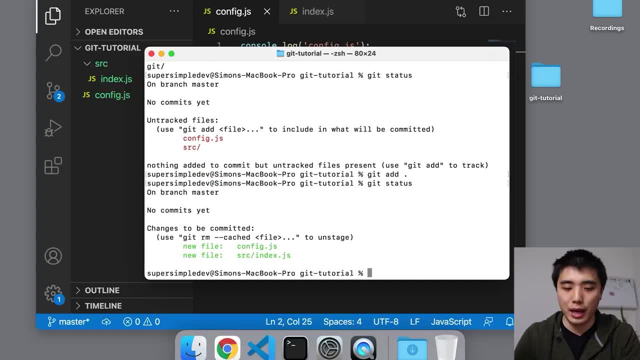 if you want to add everything into the next version. So we're gonna press enter to run this command, And now we're gonna run git status again to verify that it worked. So now you can see we have two new files that are ready to be put in our version history. 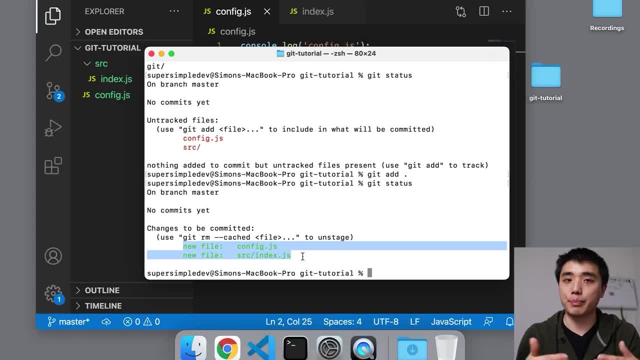 So remember that git add doesn't actually create a new version. It just lets us pick which changes we want in the next version. So to create a new version we're gonna use another git command, which is git commit dash m. So a version in git is known as a commit. 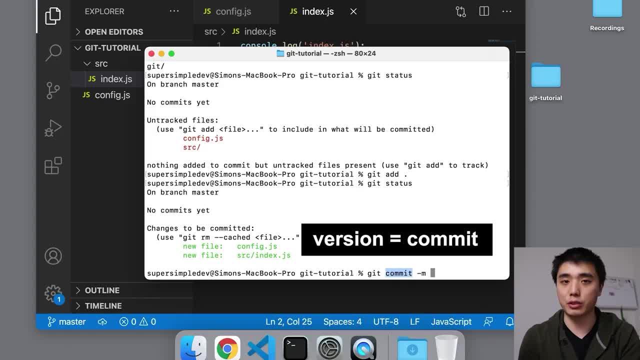 As this tutorial progresses, I'm gonna be using the words commit and commit history instead of version and version history, just to help you get familiar with the git terminology. But for now I'm gonna use version, just because we're comparing with the Google Docs version history feature. 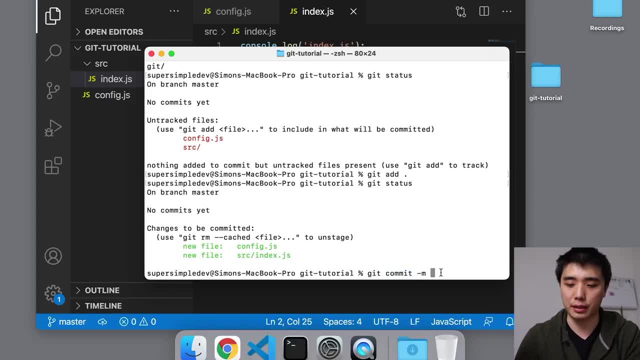 So dash m here means we are attaching a message to this commit. So you always wanna attach a message to a commit just to describe what you changed, so that when you're looking at this commit down the road you'll know exactly what happened. So, since we're just practicing, 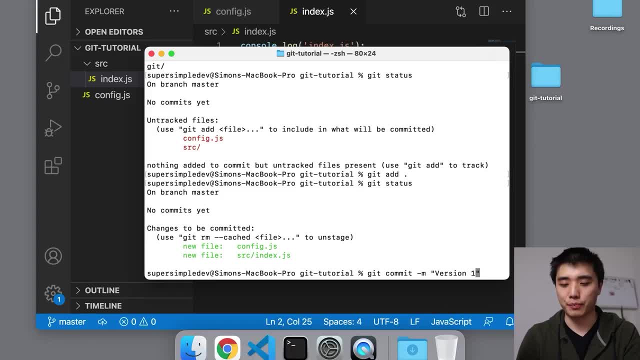 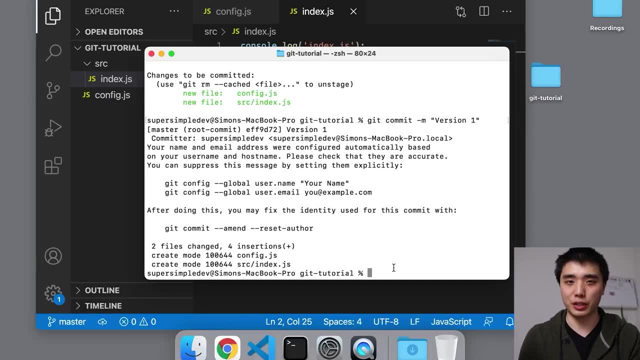 I'm gonna give a very simple commit message, version one, And to run this command we're gonna press enter And that's it. We just created the first version in our version history. So I realized that, depending on your computer, you might actually get an error message. 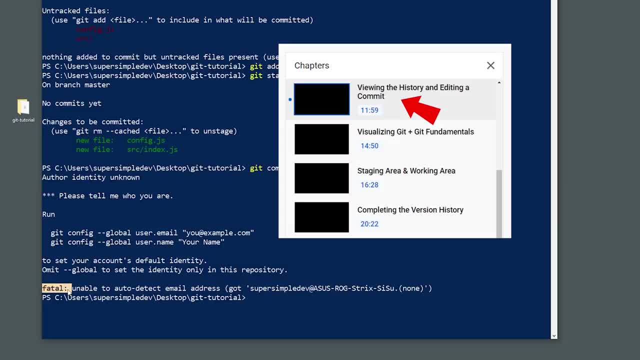 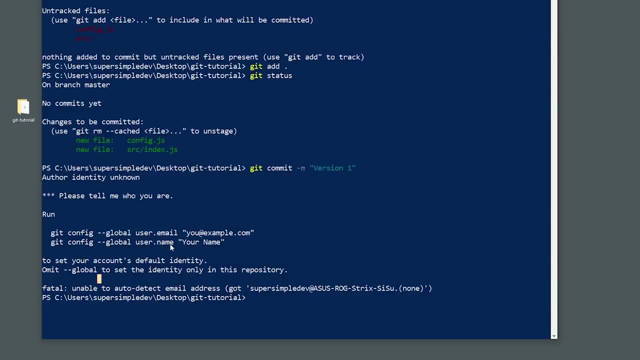 that looks like this fatal. If you didn't get an error, then feel free to skip ahead. So this means that git is requiring you to do this. It's requiring you to configure an email and a name to git that will be attached to your commit. 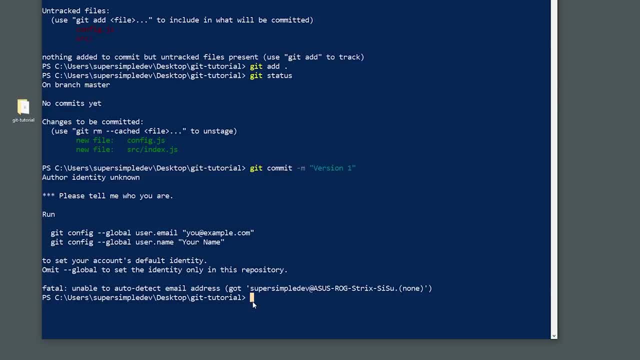 along with your commit message. So we're gonna explain right after what this means. but to get past this error you just have to run these two commands. So you're gonna run git, config, dash, dash, global useremail and then you're gonna give your email. 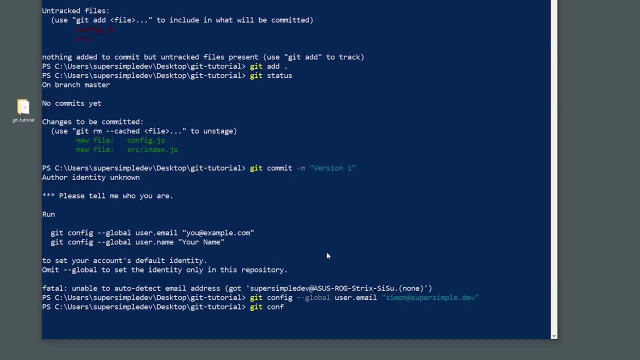 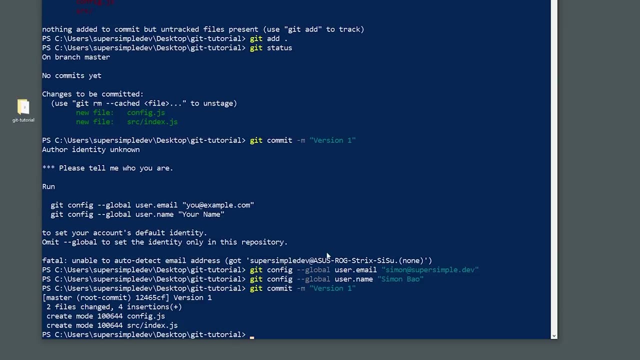 And we're also gonna configure our name. So git config dash dash global username And I'm gonna run this, I'm gonna put my name and you can put your name, And now we're gonna run git commit again, And that should work successfully. 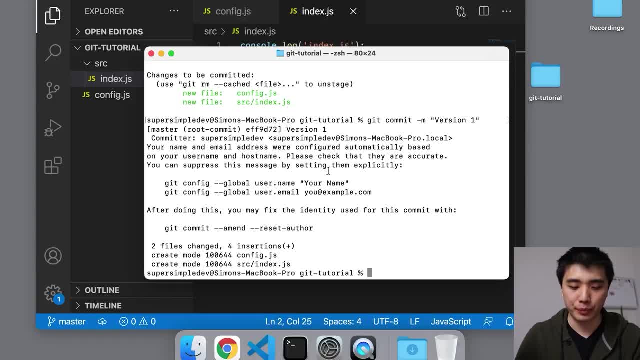 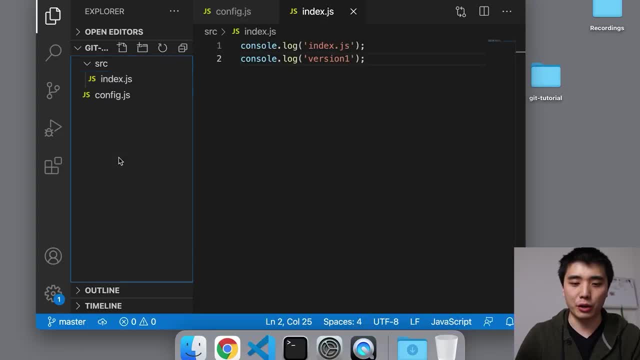 So you can see there was a lot of text output here. We're gonna go through it one by one. So in this section we're basically saying that two files were modified and there were four lines of code added. And if you look at our code, 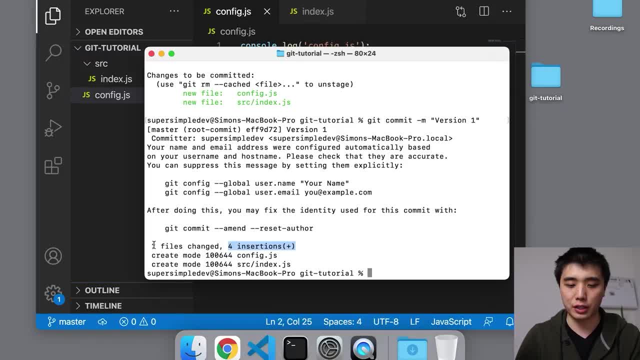 we actually do have four lines of code. So that's what this section describes, And in this section, git is basically just warning us that we haven't configured a username or an email to git. So, in addition to your message that you attach to each commit, 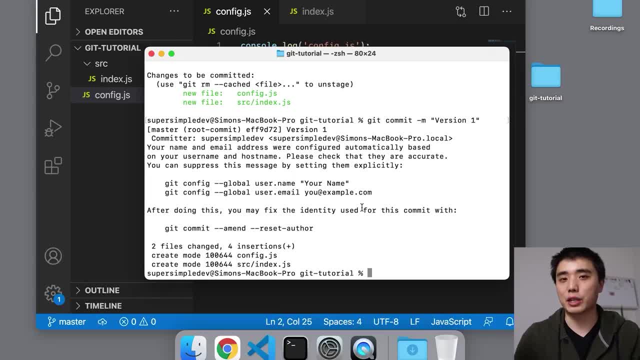 you also wanna attach your name and your email. That way, in case one of your changes breaks the website, your teammates know who to blame. So that's what we're gonna do next, And all we have to do is actually just follow these commands. 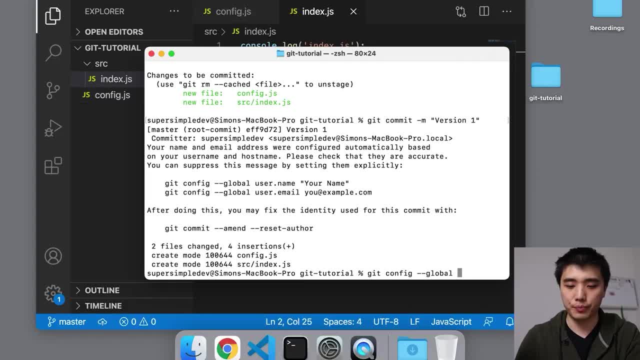 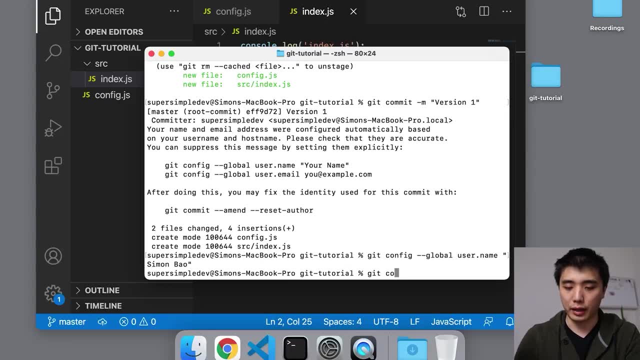 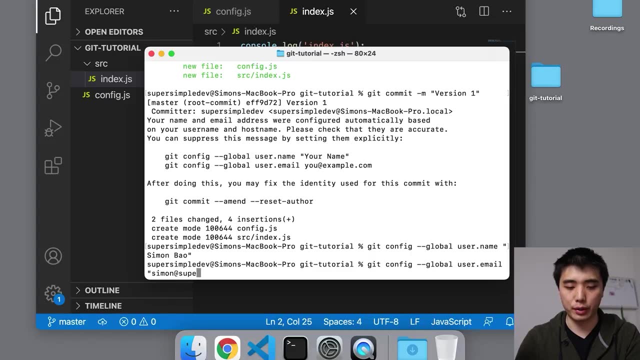 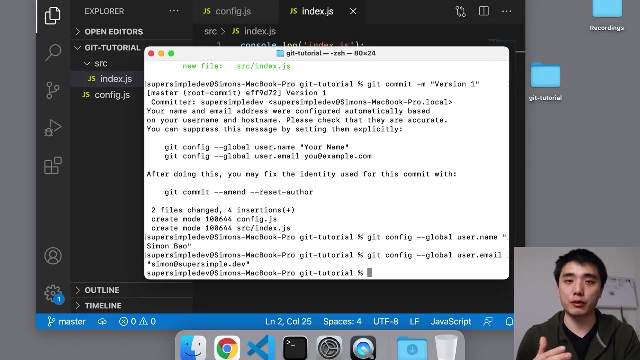 So git config dash dash global username. So I'm gonna put my name. you can put your name And git config dash dash global useremail assignment at super simple dot dev. So now that we've configured git, let's take a look at our version history. 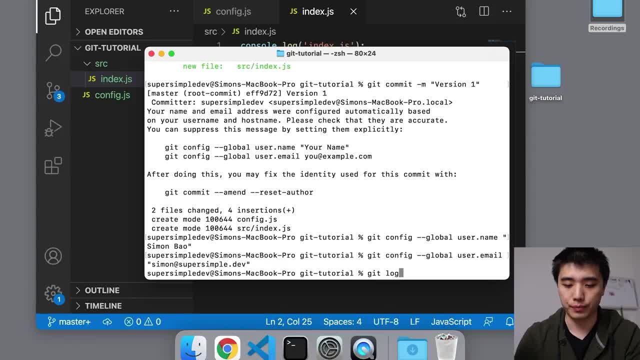 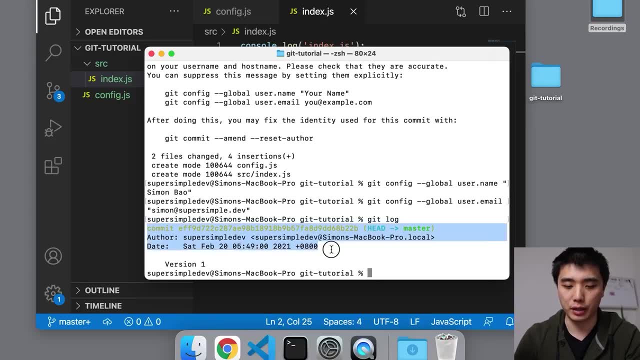 So we can do that using this command: git log. So this is our version history. You can see that we only have one version in here right now, which is the one we just created, And here is our commit message. Here is the author's name. 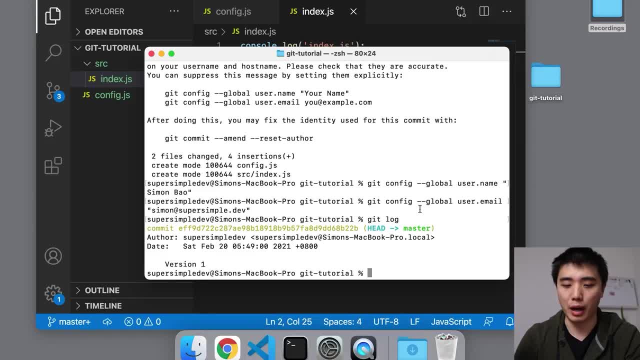 Here is the name and email. So notice that we configured the name and email after we created the commit, So that's why we have a default name and email based on my computer, And that's it. We just learned how to add new versions. 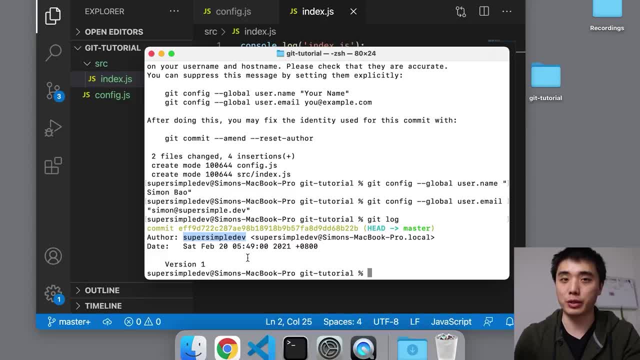 to our version history. Later on we'll learn how to go back and forth between previous versions of your code, But for now, I do wanna show you one other thing. So let's say that while you're creating this commit, you make a mistake. 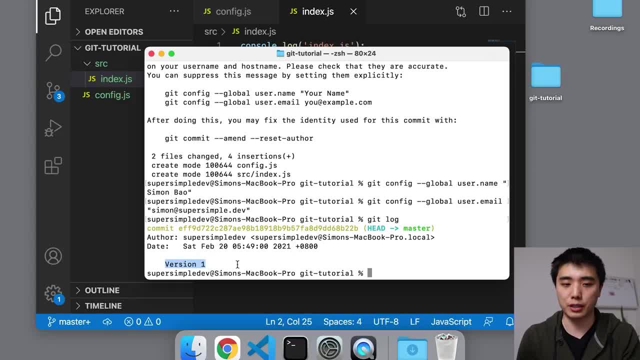 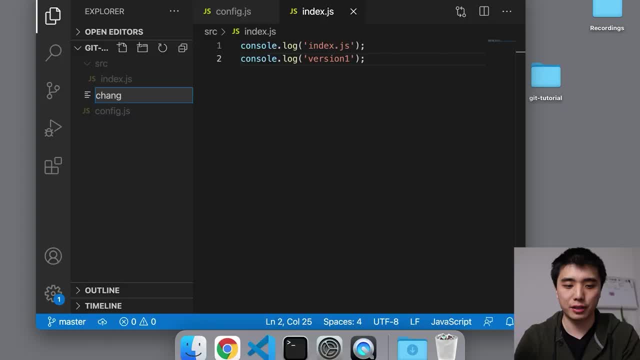 So, for example, you misspelled the commit message or you forgot to add a change. So how do we deal with that? So let's set this up and let's just add another change here- changejs- And let's say that we actually wanted this file. 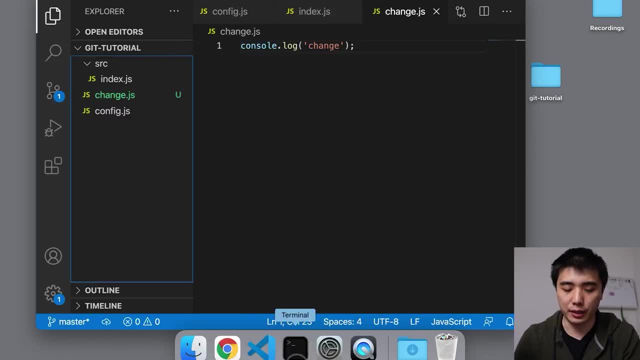 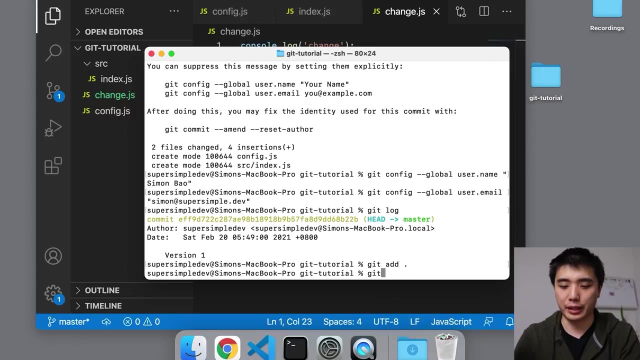 to be in our previous commit. What do we do? So the way to fix this is just to create our new version as normal. So we're gonna do git add again and git commit dash m version one. So here you can fix your spelling. 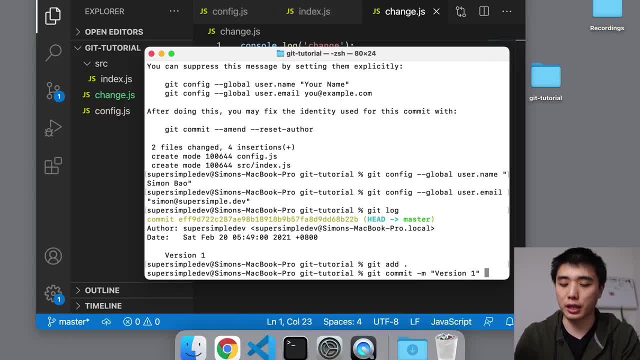 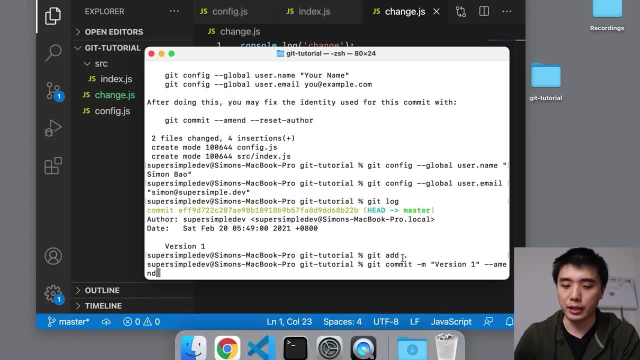 If you made a spelling mistake, And instead of just giving this, we're also gonna give dash dash amend. So what dash dash amend means is that instead of creating a new commit, these changes are just gonna go in the previous commit. So let's press enter to run this command. 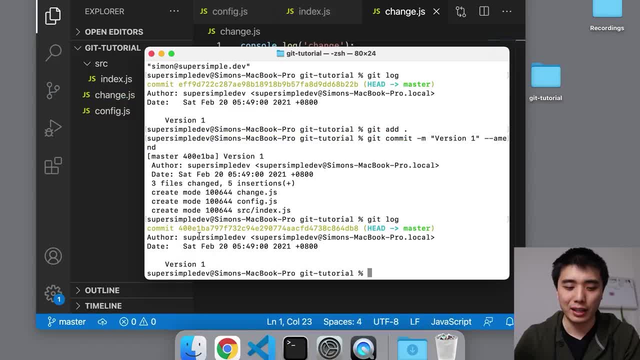 and now we're gonna run git log again. As you can see, we still only have one version in our version history, and the extra file that we created has been added to that version. So that's how you can edit a commit, including, you know. 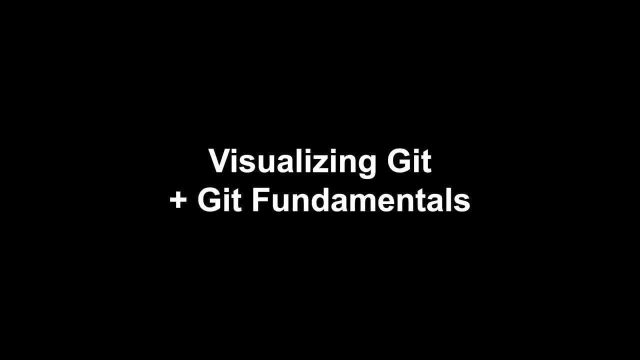 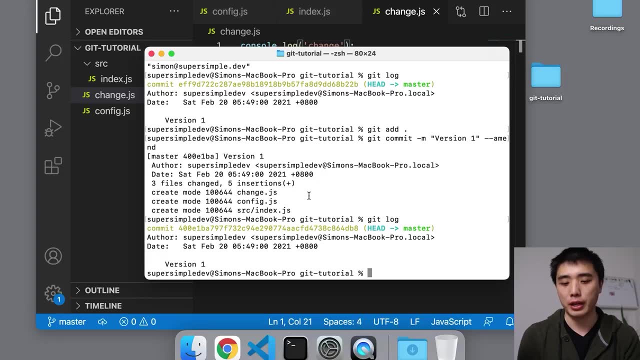 it. in case you mess up. Now I want to show you how you can visualize the changes that Git is tracking inside your code editor. So a lot of editors have Git integrations these days that allow you to see what changes Git is tracking inside your editor instead of just in the command line. 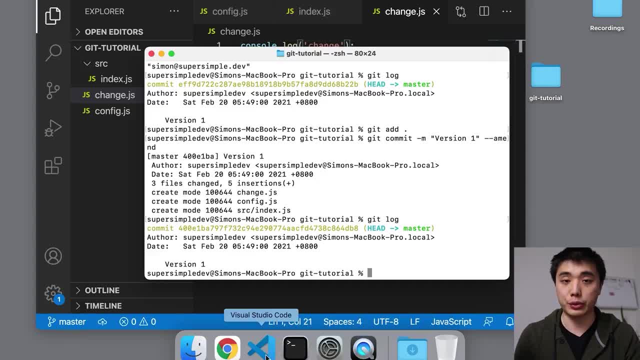 So I'll show you how that works. So the editor I'm using is called Visual Studio Code, So you might be using a different code editor, so you'll have to check if your editor supports Git integration. So in VS Code we can actually visualize what changes we have made since the previous version. 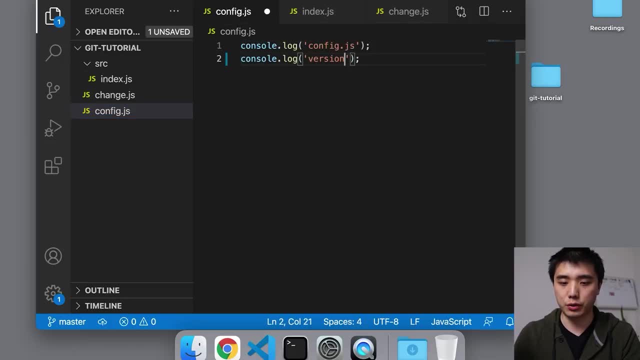 So let's go ahead and make some changes. here, I'm just going to change this to version 2, and here as well, I'm going to change it to version 2.. So now, if I go into this section- this is the Git section- we have our changes that. 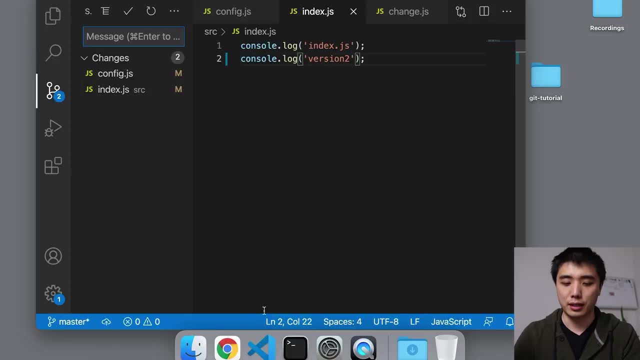 we made to Git here. So this is the same thing as running git status in the command line, except we can actually visualize it in our code editor. So if I select one of these changes, we can actually see what code we have changed in. 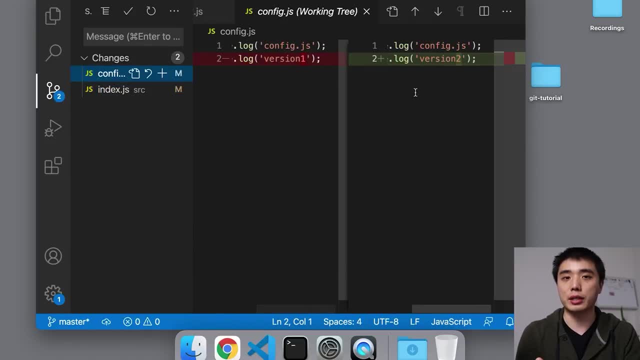 this file and also for this file. So you can see that it can be really useful if you're working on a big feature and instead of two files here you have like 20 different files and you can see exactly which code that you changed. 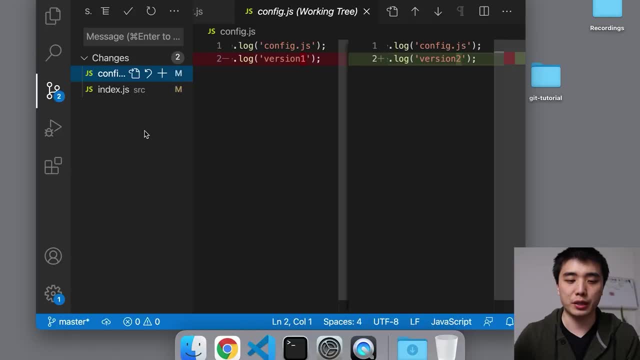 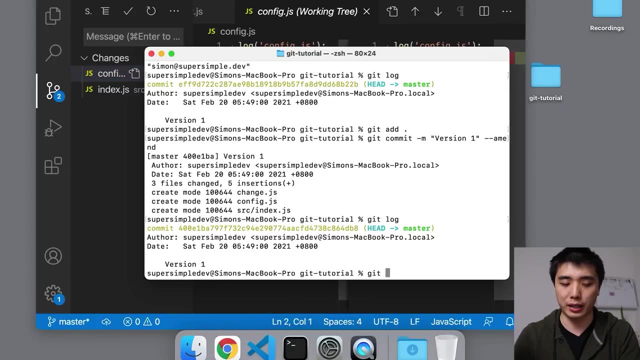 So this editor also allows us to run some Git commands for us. So, for example, if I want to git add this file, I can actually press this plus button instead of going to the command line and running git add myself. If I want to add this file, I just have to click the plus button here, and if I want 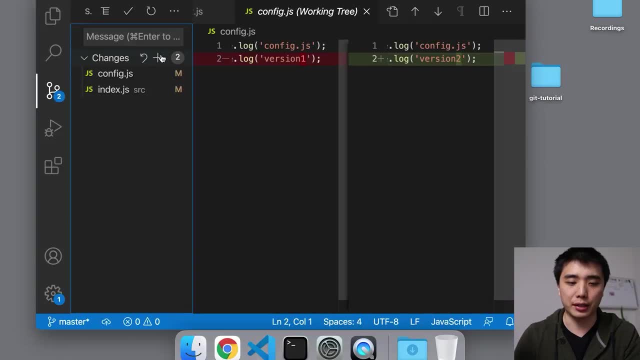 to do git add dot, then the equivalent is just clicking this button here. So it makes it a little bit easier to run Git commands just from your code editor. So you might have noticed that when we ran git add dot the changes were placed in this. 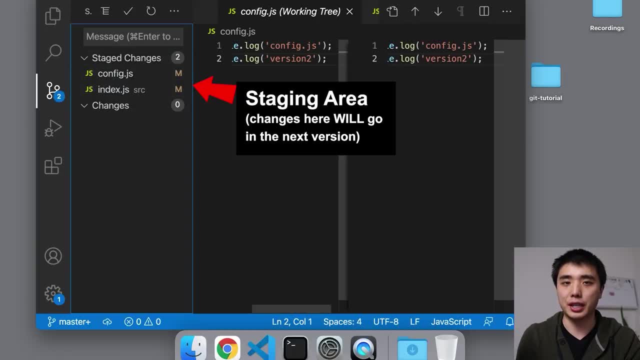 area called staged changes, So this is known as the staging area. This is basically where Git puts all of the changes that we have picked using git add that we want to go into the next version, Otherwise we might forget. And then under the staging area is all of the changes that we are currently working. 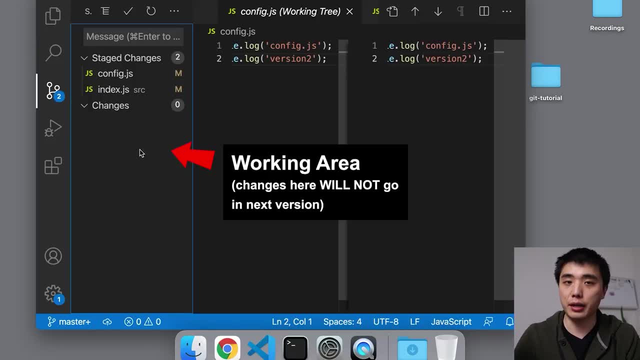 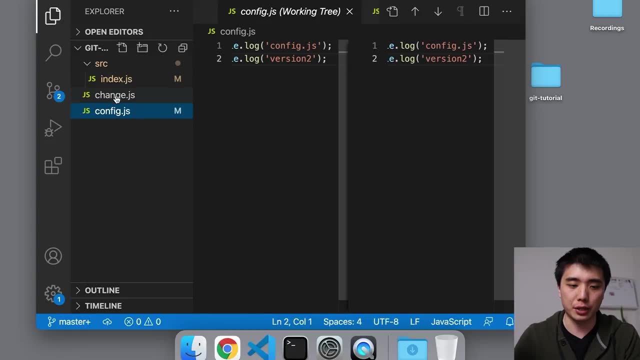 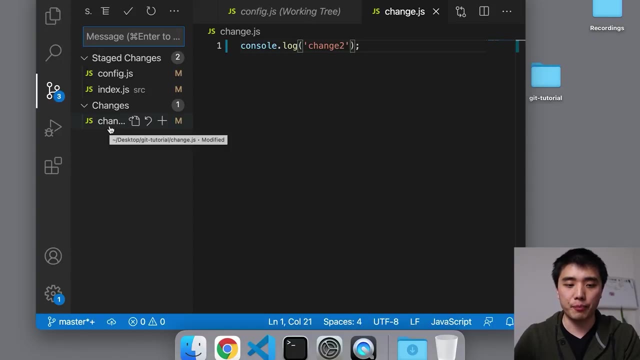 on, but we haven't used git add yet, So this area is called the working area. So all of your changes start off in the working area. So let's make a simple change right now, just to visualize it. So now you can see that that change starts off in the working area. and then, when I run, 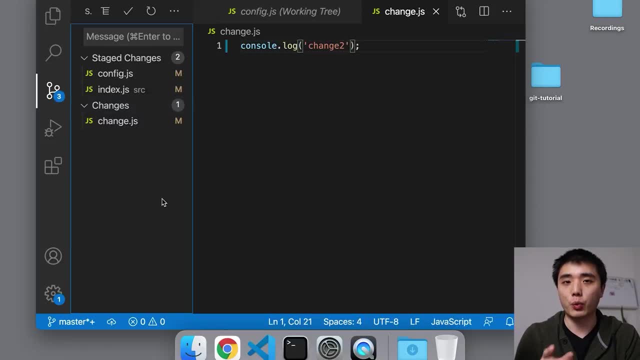 git add. it's going to add it to the staging area. So one other thing I want to show you about the staging area is that Let's say that we go ahead and modify this file again. So let's go into config and let's have another simple modification. 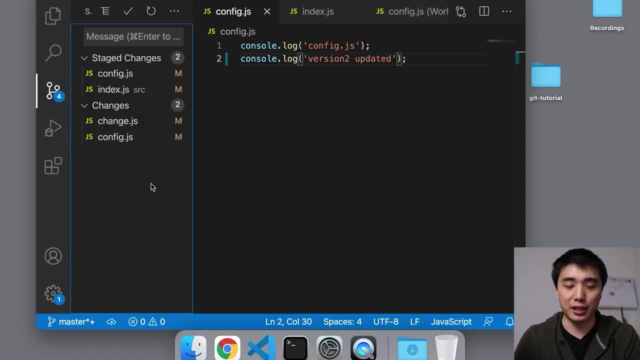 Save it. We'll go back So you'll notice that config dot js is now both in the working area and in the staging area. So how does that work? So the way that git works is that it actually tracks changes, not files. 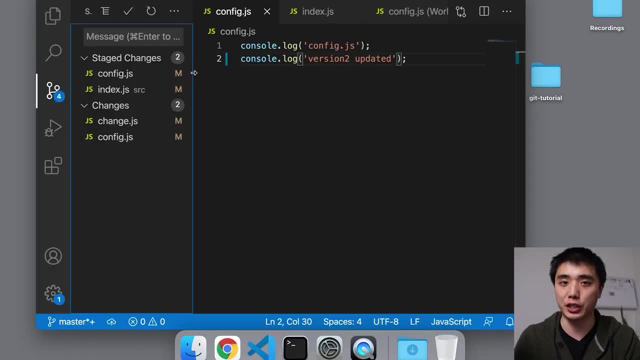 So even though we git added the file config dot js to the staging area, the second change hasn't been added yet, Because git fundamentally tracks changes, So that's why it can appear in both places. So let's go ahead and add these two files to the staging area and you'll notice that. 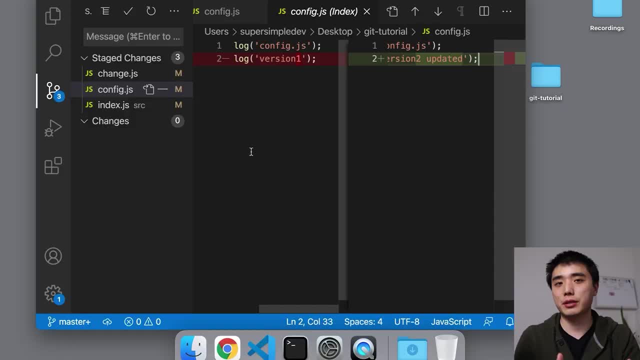 it actually merges the two changes together. So that's just some foundational knowledge about how git works. You're going to be using the staging area a lot, so it's pretty useful to know some of these facts about the staging area, as well as the working area. 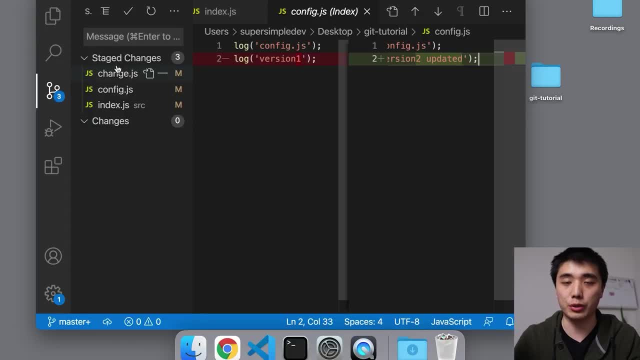 So the last thing I want to show you about these features is how to take changes out of our staging area and how to reset our working area. So let's start with staging first. So to take changes out of the staging area, our code editor might provide a convenient. 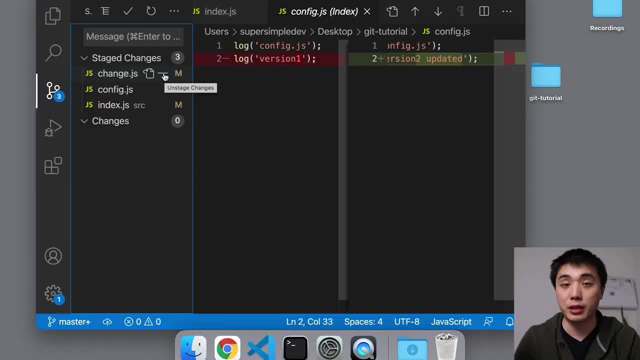 button in its git integration, and my code editor has one right here. So all I have to do is click this button and it will take the change out of the staging area. So now let's also learn the git command for doing this. 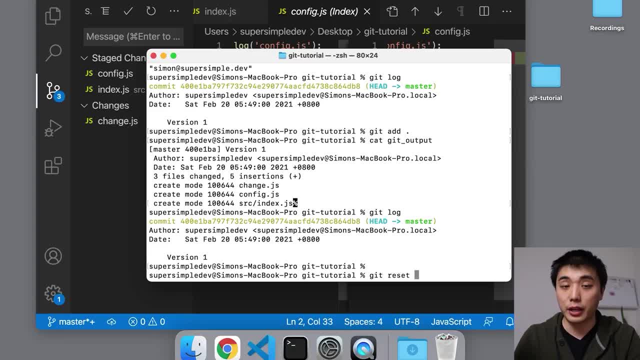 The command for doing this is git reset, So reset works the same way as add. If we give it a file name like reset config dot js, It will only take config dot js out of the staging area. If we give it a folder, it will take all of the files in the folder, including any subfolders. 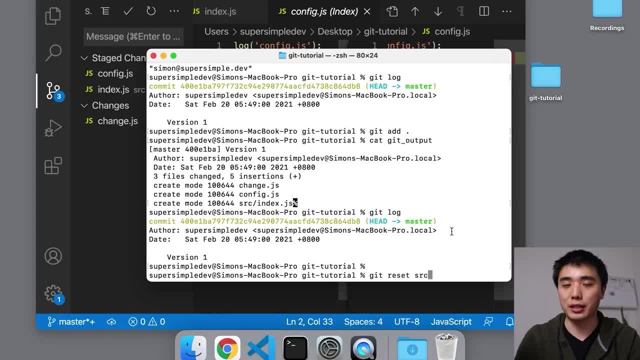 and take all of that out of the staging area. So remember, a shortcut that we can use is git reset dot. So dot here represents our current folder, which is this folder that contains all of our code. So if we do git reset dot, it will take all of the changes out of the staging area. 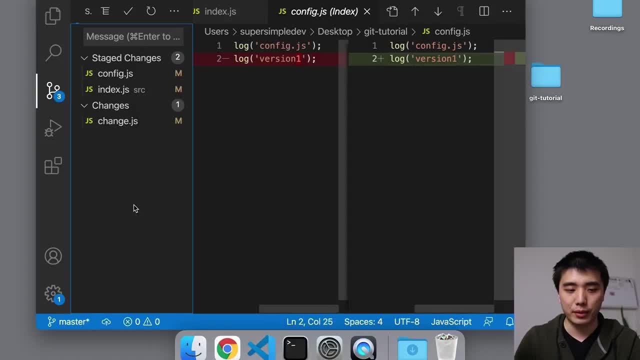 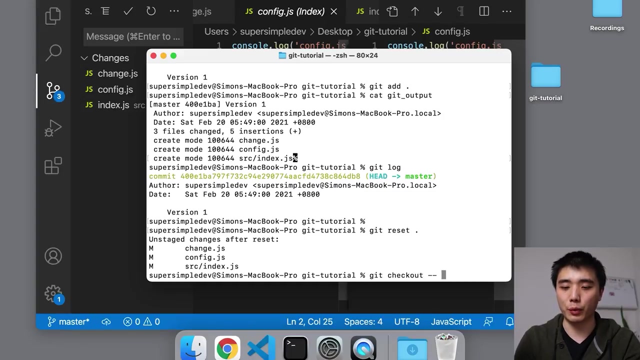 So let's go ahead and run this command. So now all of our changes are in the working area and we can also reset the changes in our working area using another git command, And that command is git checkout, dash, dash, and this works the same way as git add. and 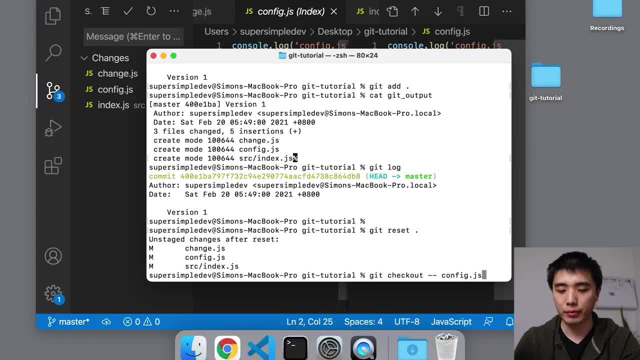 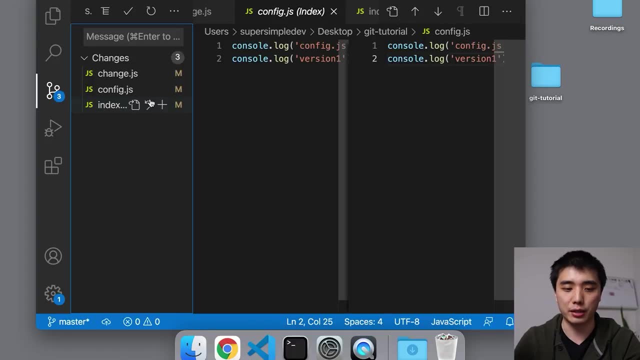 git reset. We can give it a file name which will undo all of the changes to this file in the working area, or we can give it dot, which will remove all of these changes. So for this time, Let's go back into our code editor and use the git integration to do this. 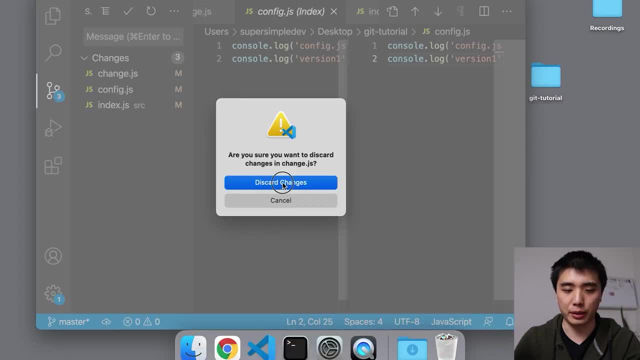 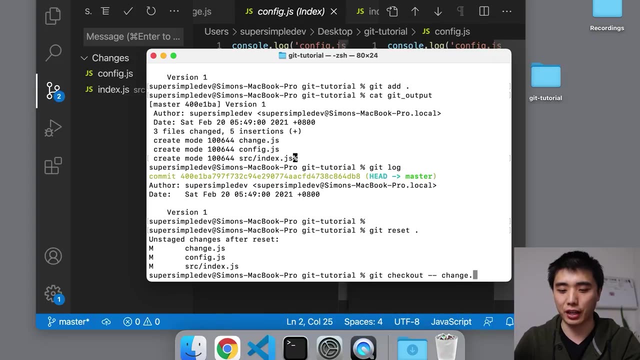 So if I click this button, this is the same thing as doing so we reset change dot js. this is the same thing as doing git checkout dash dash, change dot js. And if I click the button up here, this is the same as doing git checkout dash dash dot. 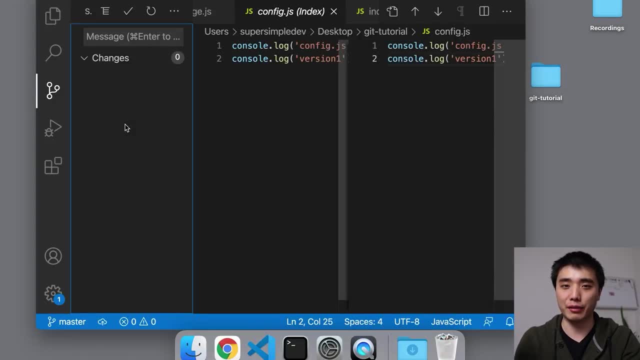 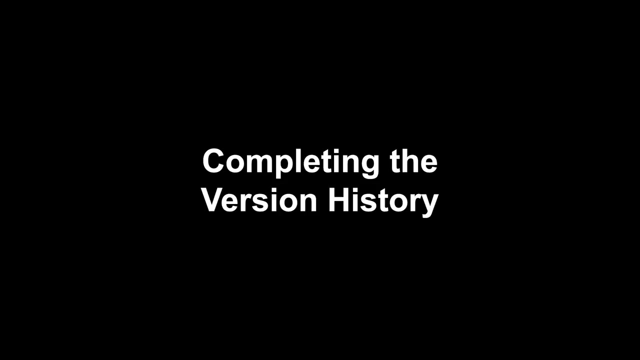 So you can see how a git integration in your code editor can really make your life easier when you're working with git. So now we're going to move on and create the other features that we find in the Google Docs version history. Now we're going to create two more versions and add them to our version history so that 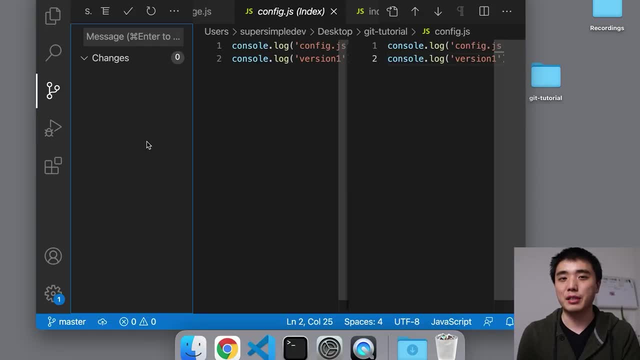 later we can learn how to go back to a previous version of our code. So if you want some practice, you can actually pause the video right now and try to create two more versions on your own. So it's the same thing that we did when we created our first version. 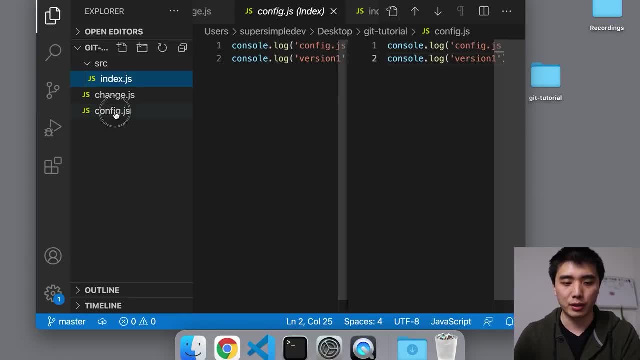 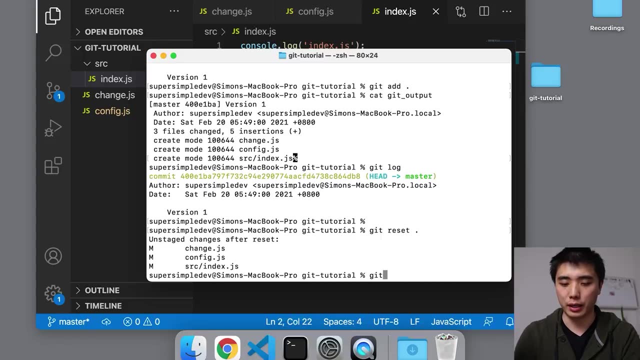 All right, so I'll do it right now for my code. So the first thing we're going to do is just make some changes, And then we will pick the changes that we want in our next version. so git, add, dot, And then we're going to create the commit with a message. 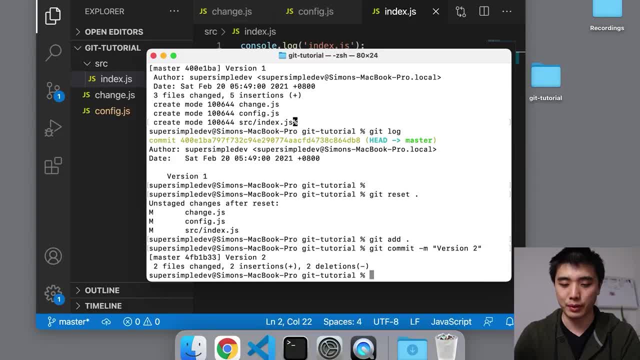 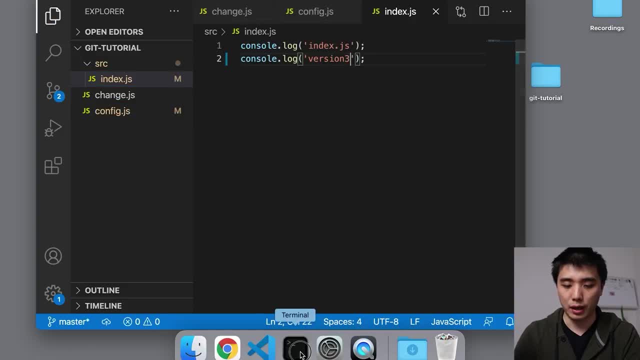 I'm just going to call this version two, just because we're practicing. Now I'm going to create another commit or another version by first modifying the code. I'm going to add the changes that I made and I'm going to pick these changes to put. 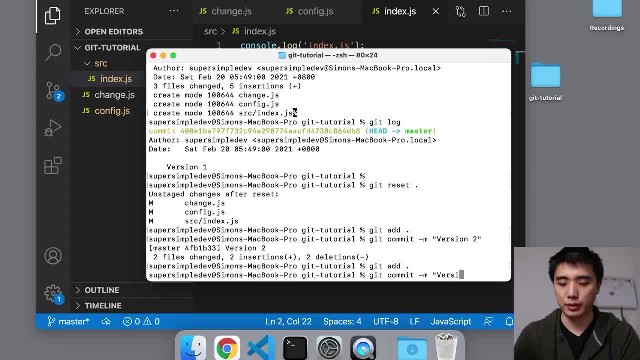 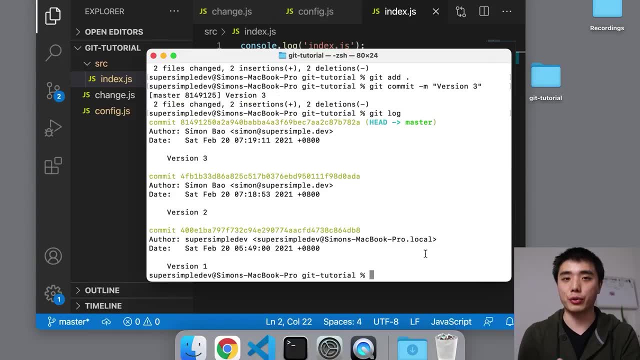 in the next commit, Then just create another commit with git commit. And now, if I run git log, you'll see that we now have three versions in our version history and now we're ready to learn how to switch between different versions. So you might have noticed that one big difference between Google Docs and Git is that Google 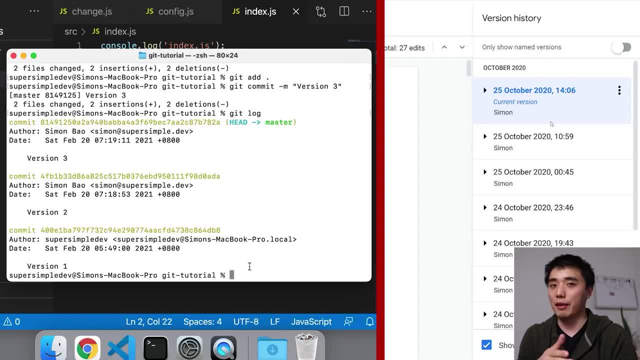 Docs automatically creates versions of your document for you, So every once in a while it'll save a version and you can go back to it later. But for Git, however, You might be wondering why are we still creating our versions manually? 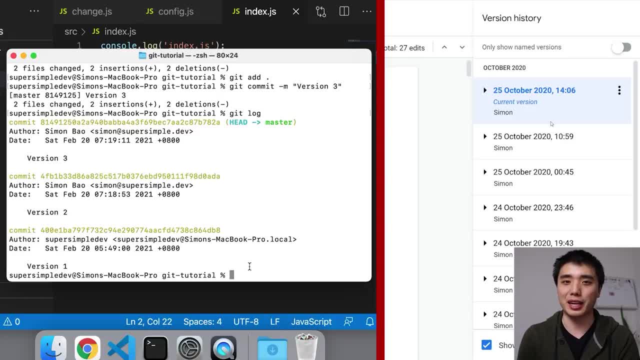 Why can't we automate this? So the problem with code is that until you finish your code, it probably doesn't work. So we don't really want to be automatically creating versions of our code that don't work. And for Google Docs it doesn't really matter if the thing's finished or not. 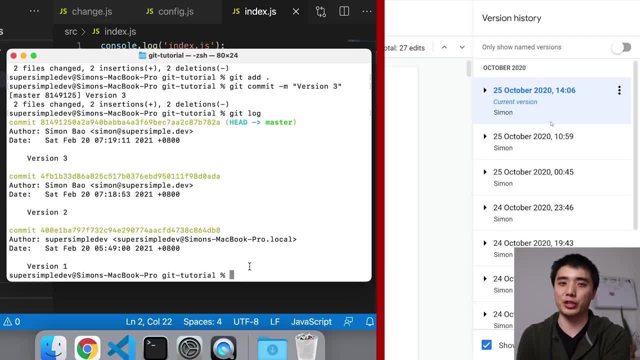 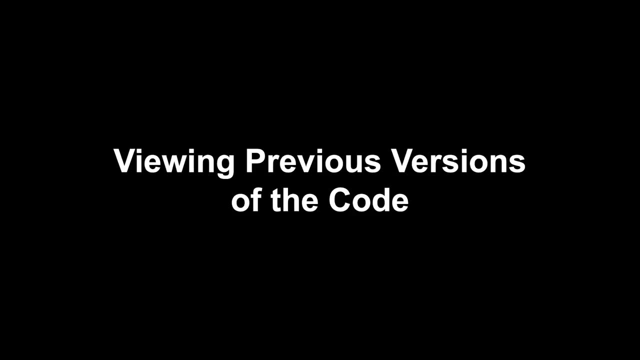 It's just a bunch of words and sentences, so you're not going to get errors from a half-finished document. That's not the same with half-finished code, so that's why we always create versions manually with Git. We want to make sure that our code is good to go before we put it in our version history. 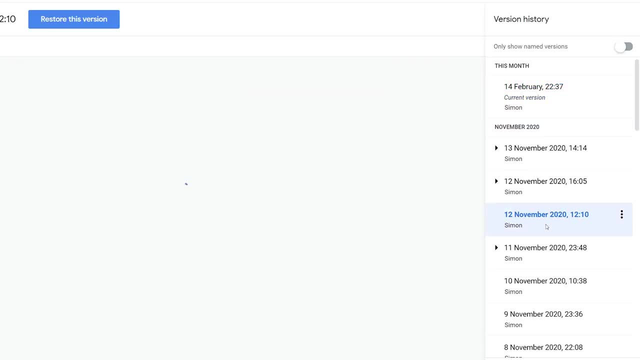 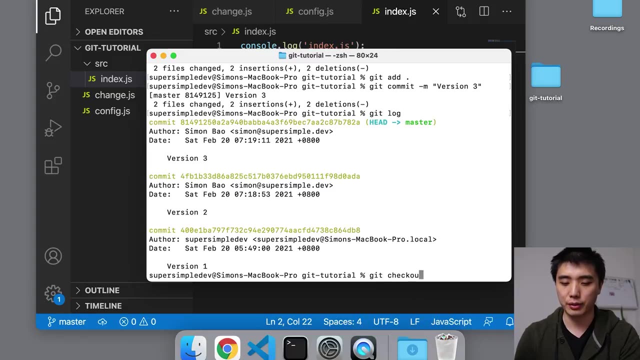 So now that we actually have a version history, we're going to learn how to go back and view a previous version of our code. So the git command for doing that is git checkout, And now we have to tell Git which version we want to go back to. 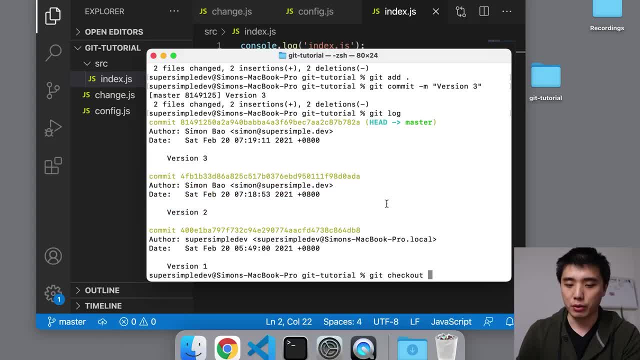 So let's say that we want to go back to this version, version 2.. So in order to tell Git that we want to go back to this version, we have to give it the this big long string. So this is known as the commit hash. 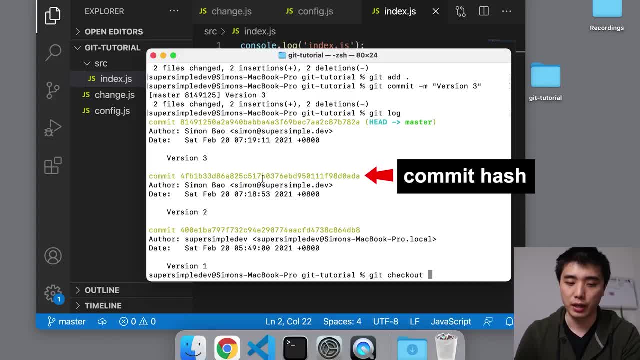 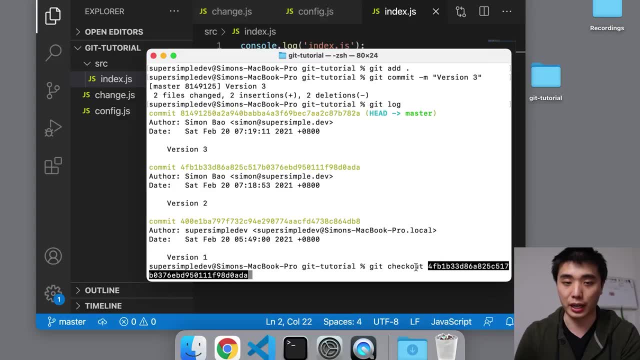 It's basically the ID of this commit or this version. So what we'll do is we're going to copy this commit hash and we're going to paste it to git checkout, And that's it. Now, if we run this command, we are back to version 2.. 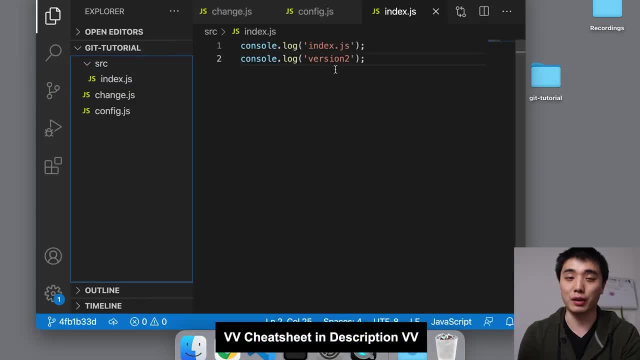 So if we look at our code, you can see that we are back to version 2 of our code, And that's as simple as it gets. We just have to run git checkout and we'll go back to a previous version of our code. 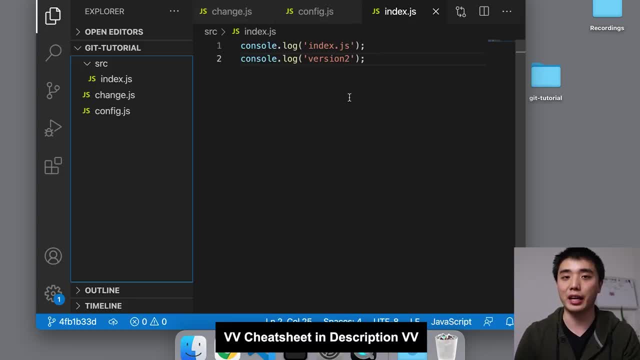 So the changes we made are really simple, but you can imagine that if we had a big feature where we changed 20 or 30 different files, this is really powerful for changing all of those files back to their previous version. Now let's go back to our command line and we're going to run git log to check the state. 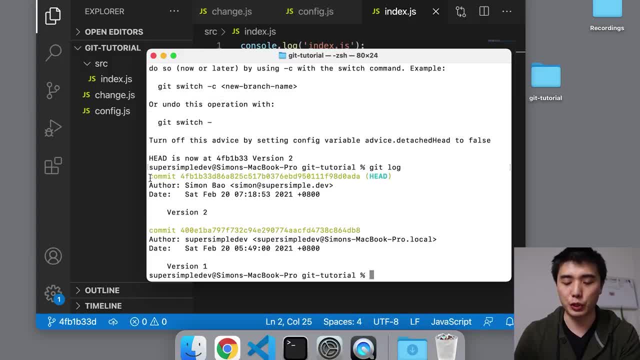 of our version history. So, as you can see, we only have two commits here right now, And the reason for that is that git log only shows the current commit as well as all the commits behind the current commit, But not any commits. 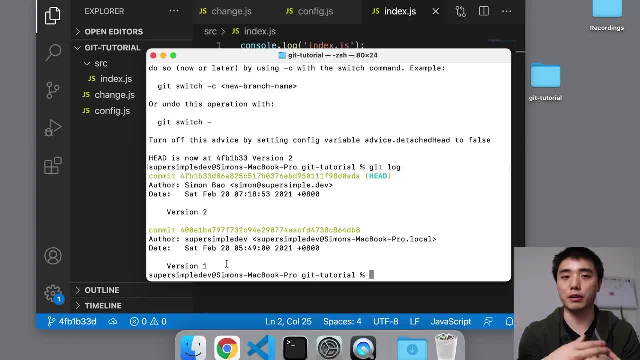 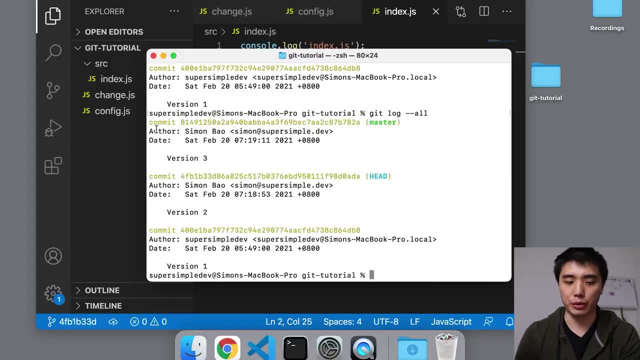 We only have the commits in front of it. So in order to show all of the commits in our version history, we're going to do git log, dash, dash all, And that will show you the three different versions that we had earlier. So you might notice that this word head is now beside version 2.. 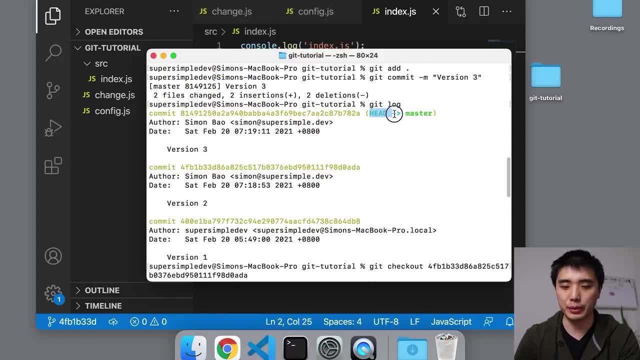 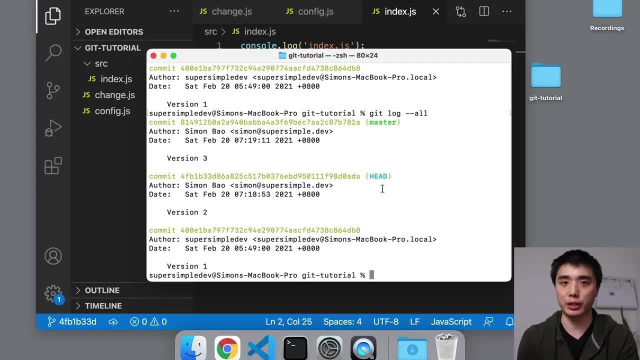 So if we scroll up to our previous version history, we can see that head used to be beside version 3.. So this word head here. this is telling us which version we are currently viewing. So in Google Docs, when you're viewing a previous version, that version will usually just be. 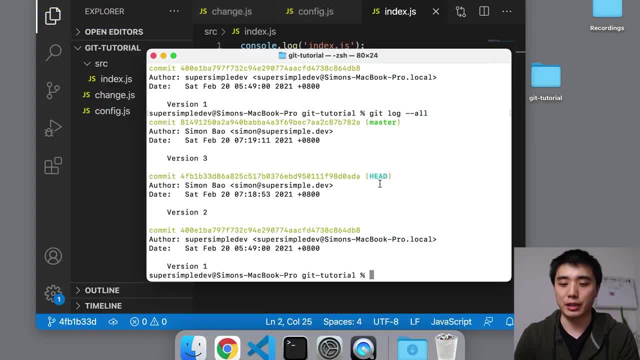 highlighted. But in the command line we can't really highlight stuff, so that's why we use this word head to indicate which version we are currently viewing. So now let's get a little bit more practice. We're going to switch to the first version that we had in our version history. 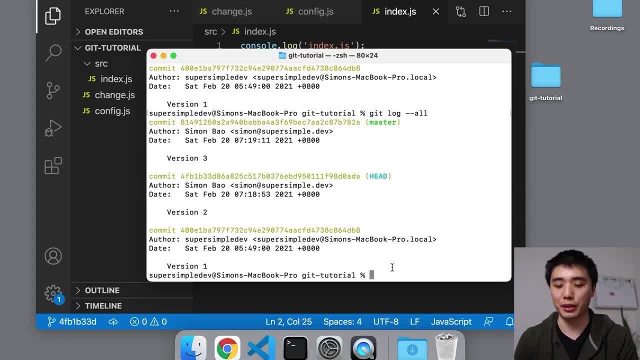 So pause the video if you want to do it yourself first, but now I'm going to do it together. So the command that we need is git checkout, And remember we need to tell git to check out. So we're going to do that. 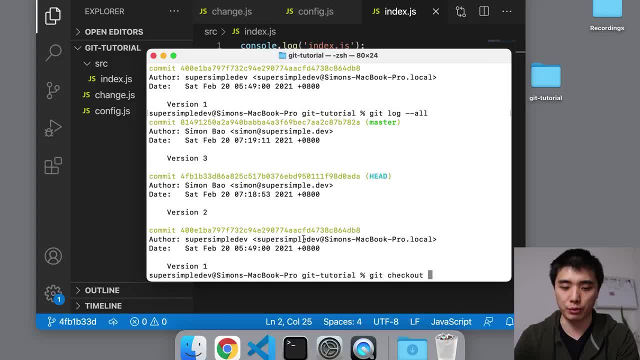 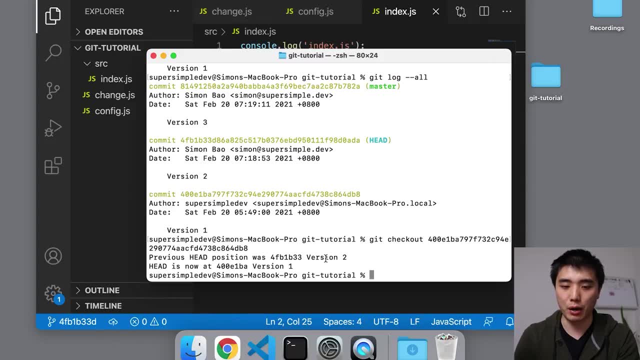 And remember, we need to tell git the commit hash that we want to go to. So we're going to copy this and paste it here, And then we're going to run this command. So now we are on version 1.. If we check our code, we can see that, indeed, our code is back to version 1.. 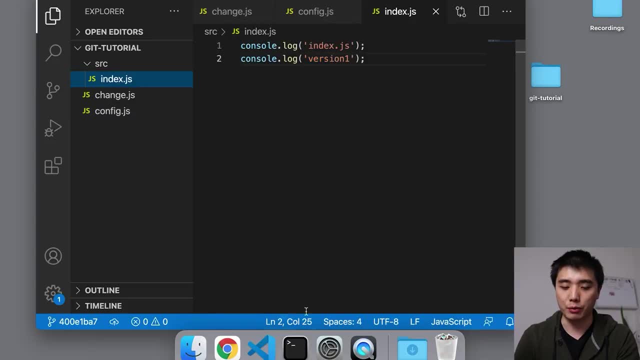 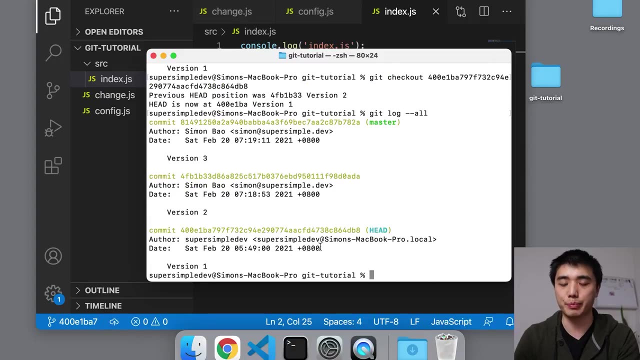 And we can check the other file. Both of our files are back to version 1.. And if we go back and we run git log, dash, dash, all we see that head is now beside our first version. So that's how you go back. 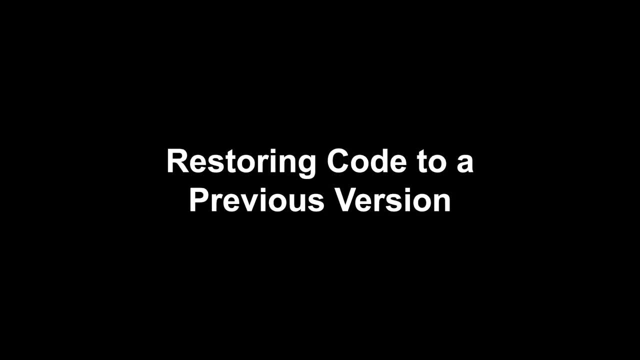 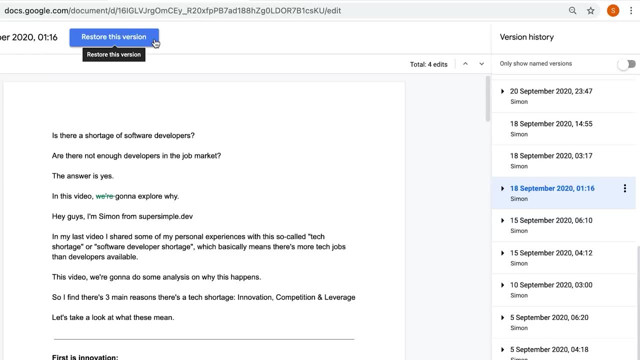 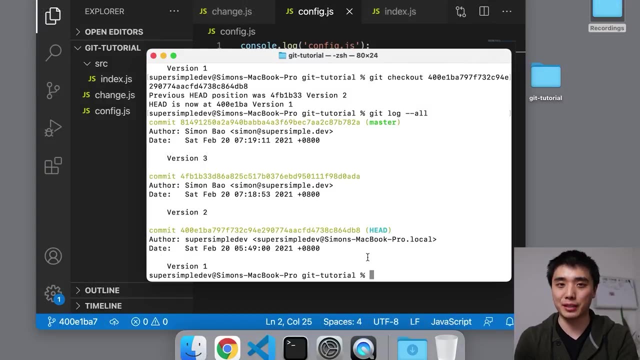 And if we go back and view previous versions of your code, The last feature we're going to recreate from the Google Docs version history is the restore this version button, which will restore the document back to a previous version. Let's learn how to do that feature except using git. 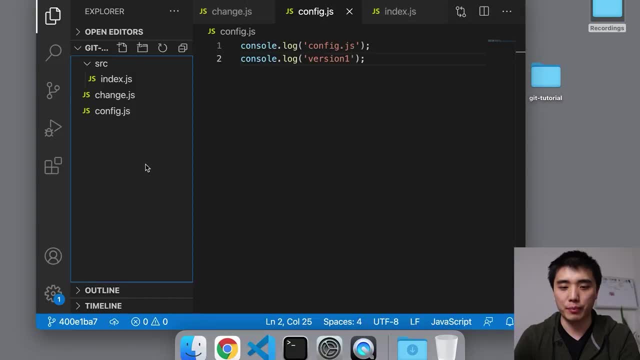 So one thing that we might be tempted to try is that we'll look at our code and realize that we've already been restored back to what it was at version 1.. So we think all we have to do is start modifying it And creating new versions, as usual. 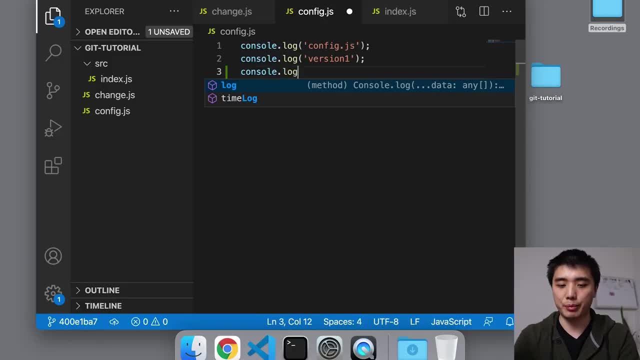 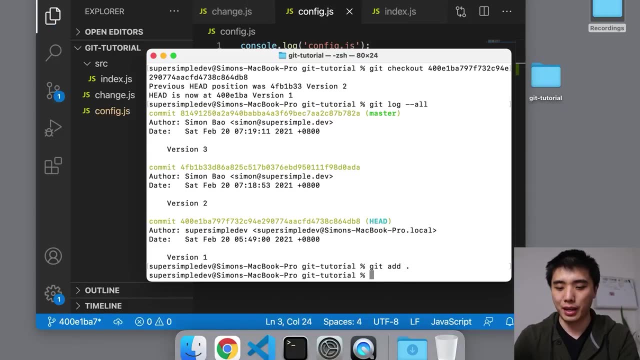 So let's give that a try and see what happens. So I'm going to do a simple update here And then I'm going to do the usual git add And then create a new commit on top of the version 1 commit. I'm going to call this version 1 updated. 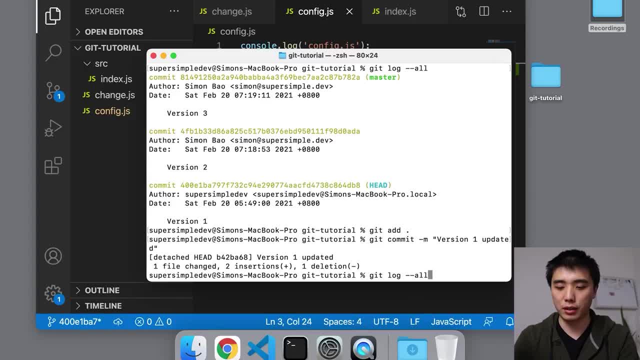 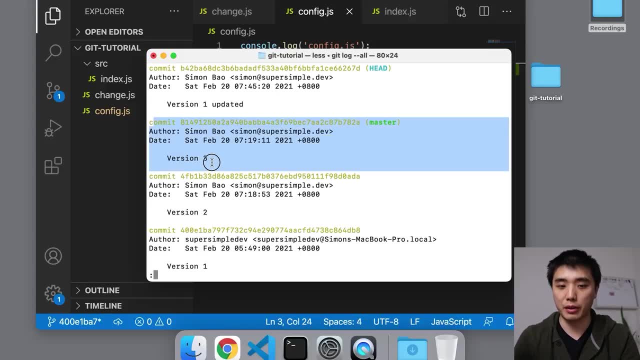 And now if we run git log, dash, dash, all, we can see that everything appears to be working fine. We have our old version 3 commit here And we now have this new version 1 updated at the top, And this one was built off of this one. 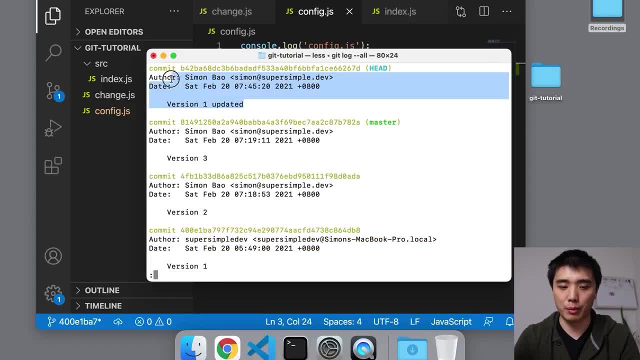 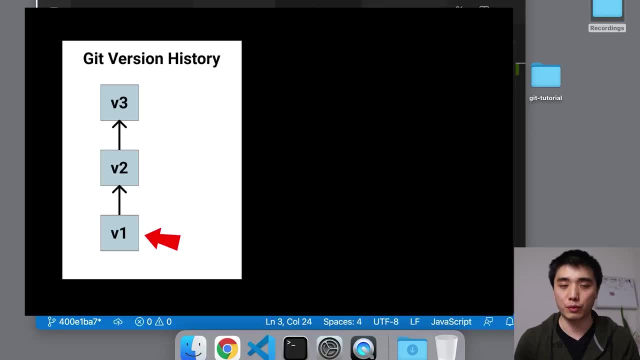 So we restored our code back to version 1.. And then we restarted from version 1.. Unfortunately, this is not exactly what we want. So the way that git works is that if you go back to a previous version and you start adding new versions on top of that previous version, you'll notice that the git history is going. 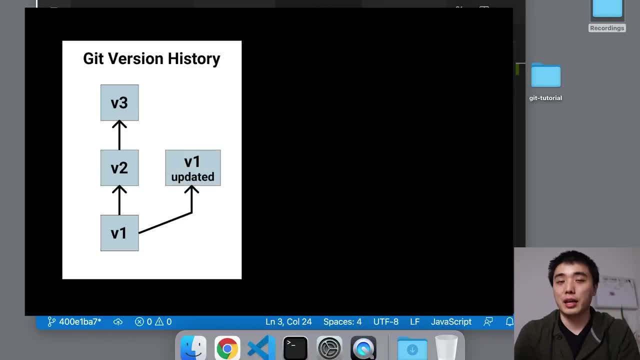 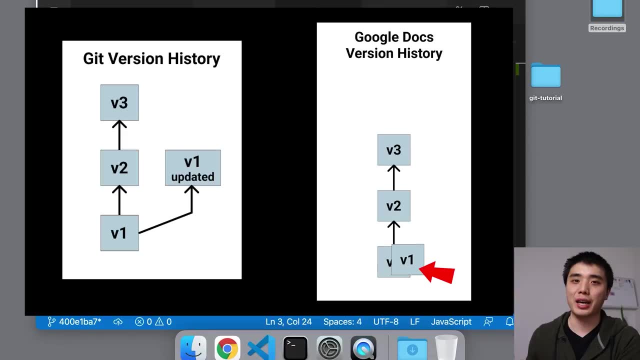 to start branching off of that previous version, And this is not the way it works in Google Docs version history. Google Docs basically takes whatever your document was at that time and then just copies it over to the current document. So this is not exactly what we want. 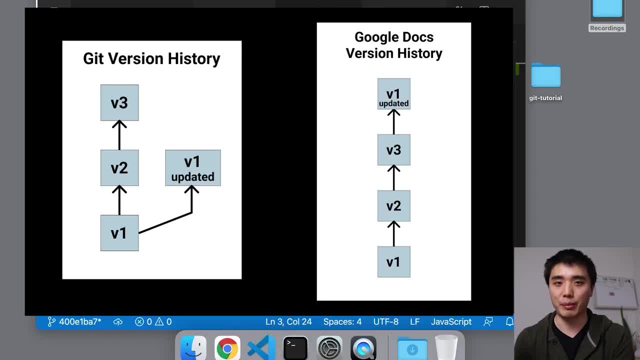 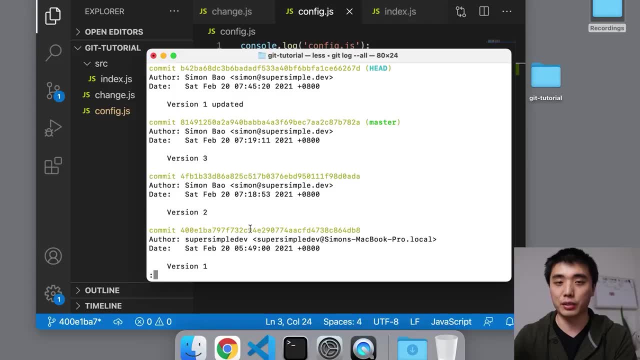 Now I do want to show you how you can view the branching effect in your command line, And you can do it with another command. So the first thing you'll notice is that we're no longer in the command line because the git log is way too long. 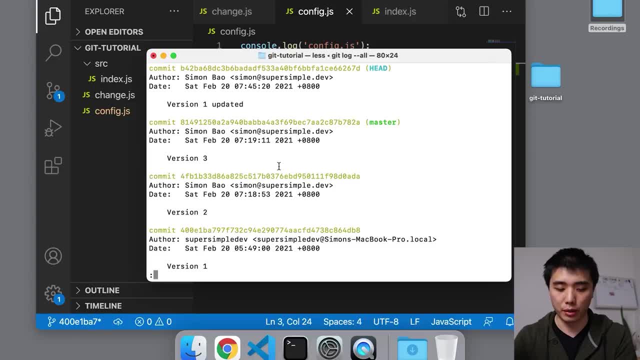 So if you try to type a command here, it won't work. So to exit out of this view, we're going to press q forward For quit. And now we're going to run git log again, except this time we're going to add dash. 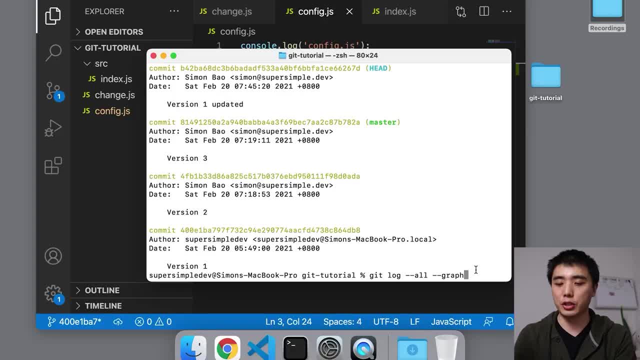 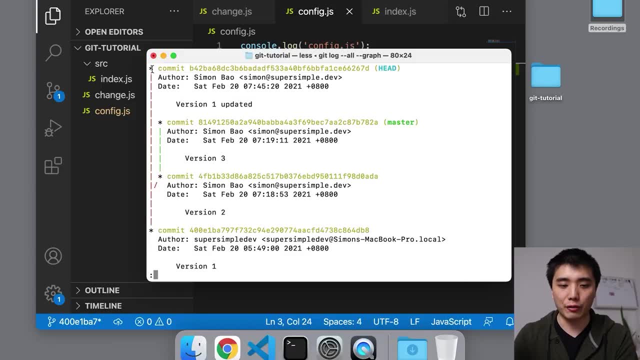 dash graph. So if you add dash dash graph, it's going to start showing you the branching effect in your version history. So we're going to run this command And now you can see we have two branches of commits. So the first branch is here, which is what we had earlier. 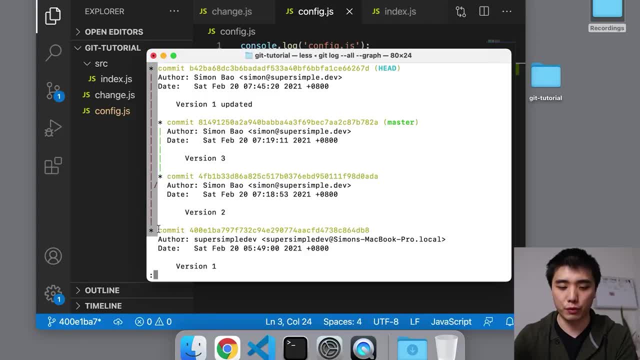 And now we have this second branch, which is built off of our first version, And this is what happens when you simply go back to your previous version and then you start building off of that version. So this is a feature in git called branching, and we're going to learn a lot more about. 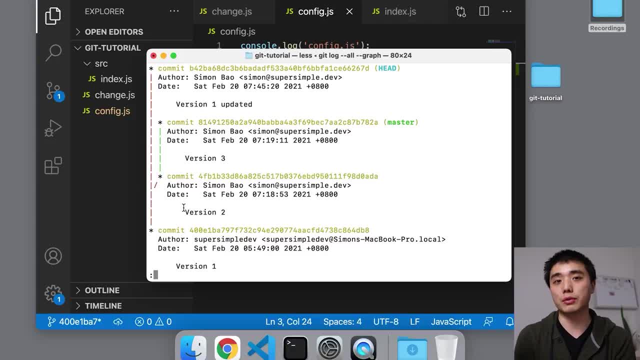 branching later, But for right now, since we're trying to recreate Google Docs version history, this isn't exactly what we want, So let's quit out of this view by pressing q, and we're going to learn the actual command for doing the exact same thing that Google Docs does. 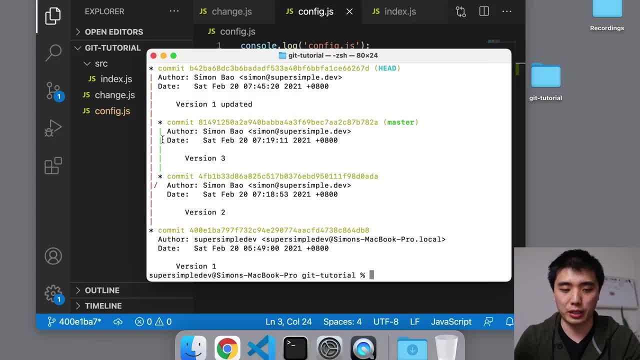 The first thing we're going to do is we're going to go back to the previous branch of commits, which is here, So you'll notice that this commit also has a branch. So we're going to go back to the previous branch of commits, which is here. 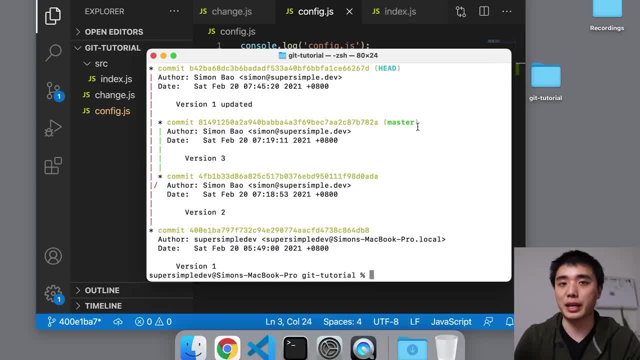 And it also has a word beside it. Mine is called master. Depending on which version of git you have, it might also be called main, So this is known as a branch name, And branch name helps us in two ways. The first way is that it makes it really easy to switch to another commit. 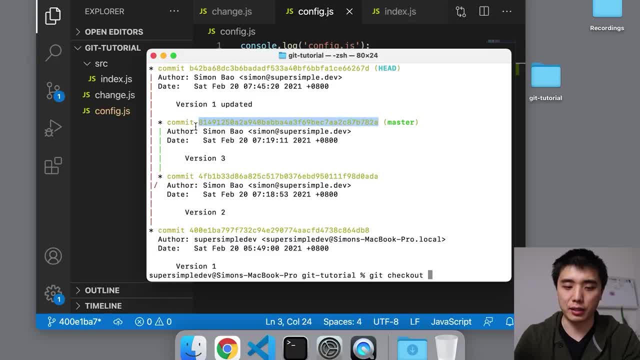 So, instead of doing git checkout and copy-pasting this long commit hash and trying to remember it, we can just do git checkout, master. And the second thing that a branch name helps us with is that it always points to the latest commit in the branch. 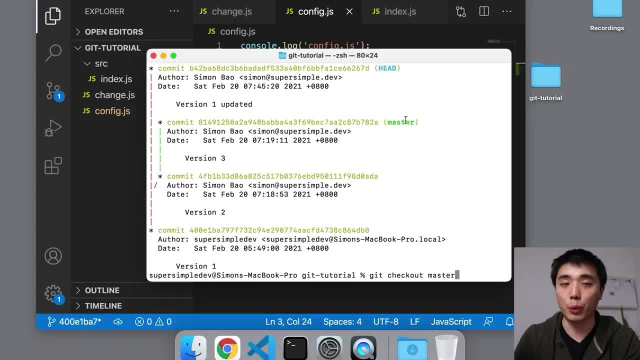 So if I add another commit to this branch up here, master will point to that commit. So this is an easy way to switch to the latest commit in any given branch. So we'll learn more about branches later, as I said, but for now just know that you. 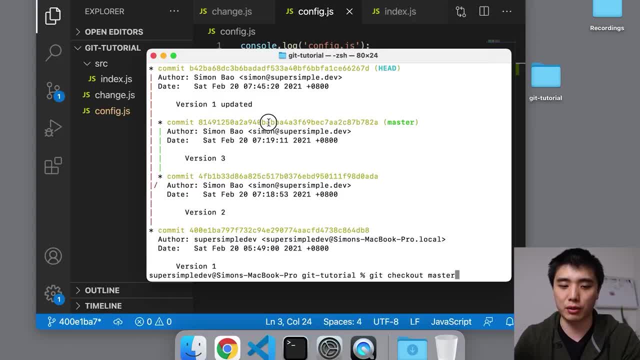 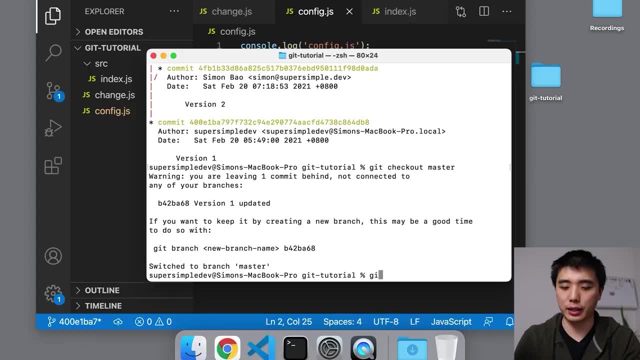 can git checkout to a branch name instead of just git checkout the commit hash. So let's run this and go back to our previous branch. And now if we run git log dash, dash, all dash, dash graph. And now if we run git log dash, dash, all dash, dash graph. 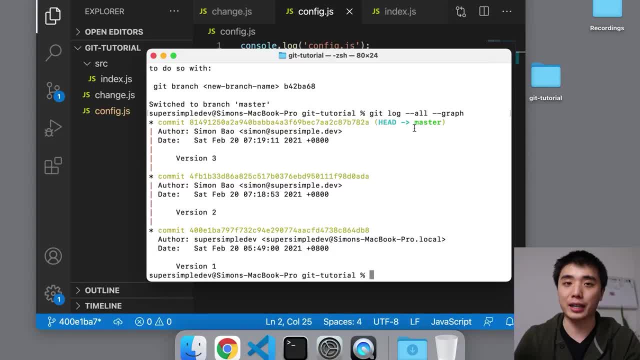 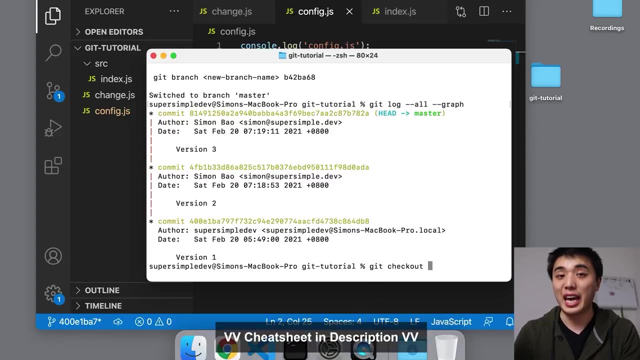 And now, if we run git log dash dash, all dash dash graph, You can see that we are now back to our main branch of commits that we had before. Now let's continue recreating that restore version feature from Google Docs. So there's actually a git command for doing this, and that command is git checkout. and 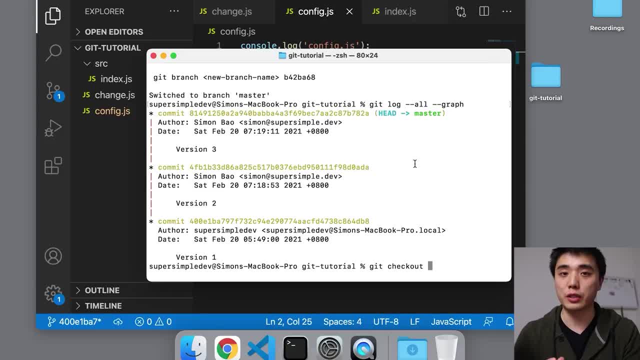 we have to tell git two things. The first thing we have to tell git is which version we want to restore from. So let's say that we want to restore from version one. So we're going to take this commit hash, copy it and paste it here. 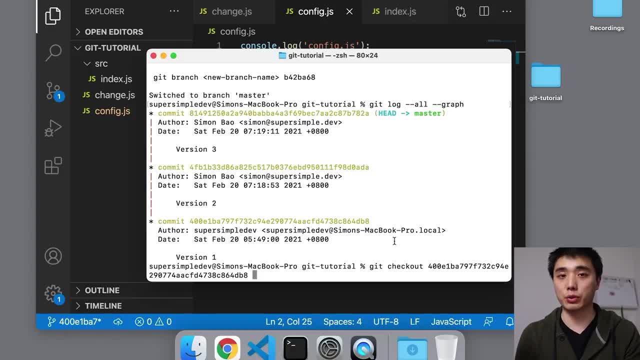 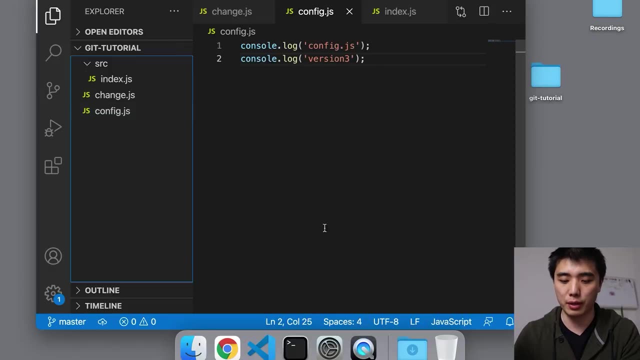 And the second thing we're going to tell git is which files we want to restore. So this works the same way as git add and git reset. We can give an individual file like this- configjs- and it will restore the contents of configjs back to what it was in version one without doing any sort of branching or 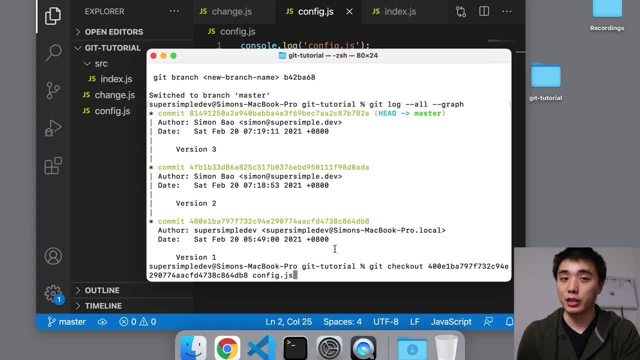 moving the head back to version one. So that's how it works. So remember: for git add, you can also give it a folder name. We can also do the same thing here. So if we do git checkout, hash and then source, it will restore all the files in the source folder. 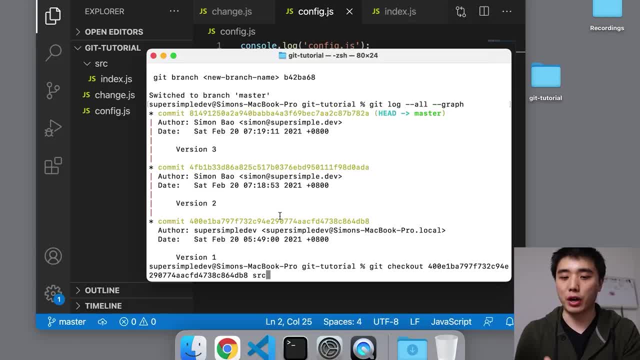 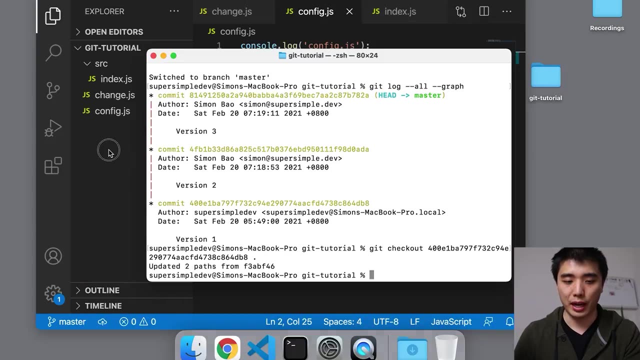 including any subfolders back to their contents in this version. So remember that we can also do dot and this will restore all the code in this folder. So let's do that. We're going to press enter to run this command and now you'll see that configjs is back. 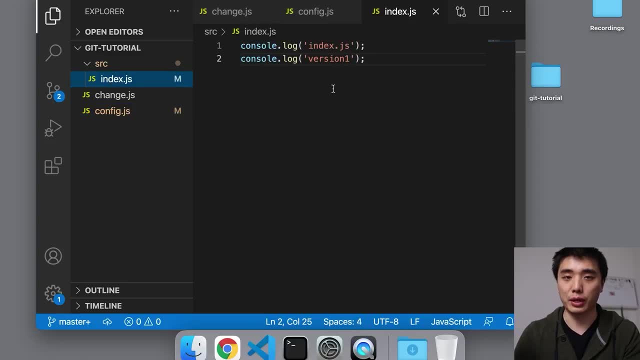 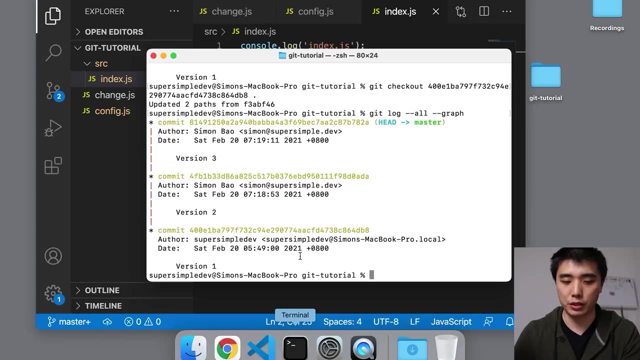 to what it was in version one And indexjs is back to what it was in version one And if we run git log, dash, dash, all dash dash graph to see our version history, you'll notice that head has not moved back to version one. 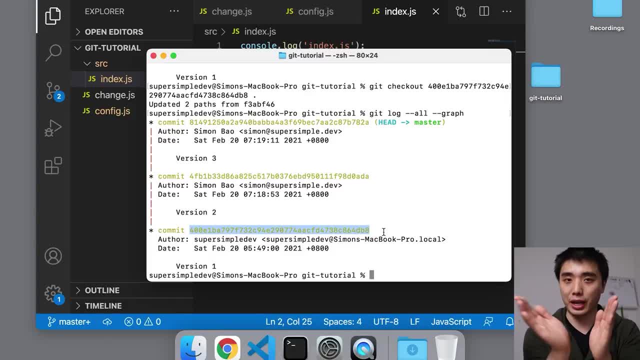 So if we add another commit onto this, it's not going to start branching our version history like we had before. So this is how the Google Docs restore version feature works: We're just taking the contents of the previous version and then putting it and pasting it. 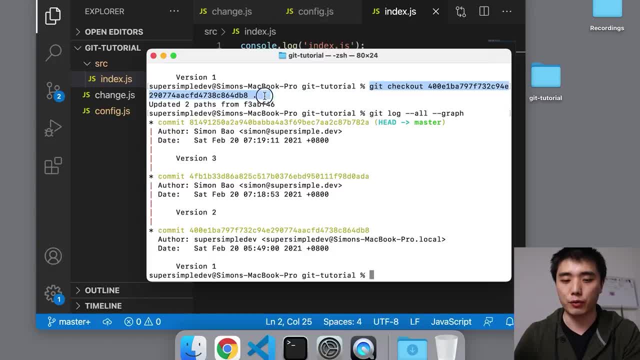 in the current version, And this is the equivalent git command for doing that. And now let's complete this exercise by adding these changes to our version history. So first let's run git status And you'll notice that when we do git checkout to restore the contents of the file to the 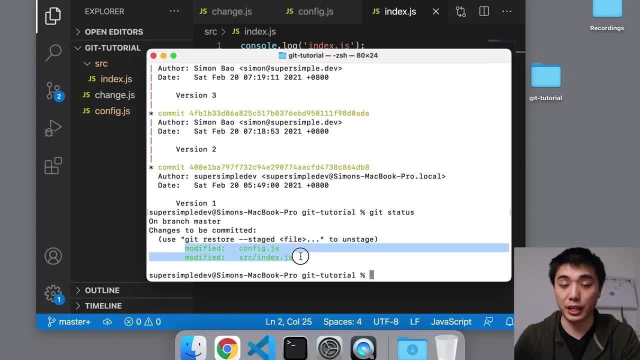 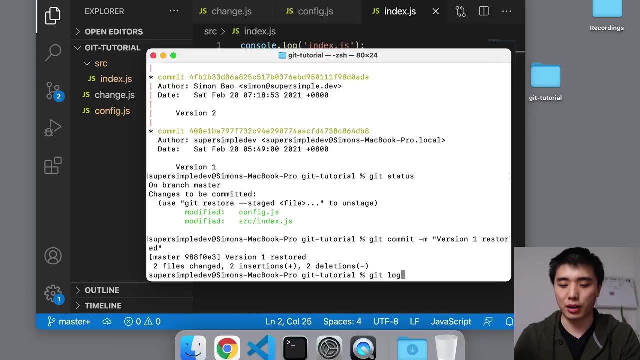 previous version. it actually automatically adds it in the staging area for us. So all we have to do is git commit dash m and give our commit message as usual. So I'm going to call it version one restored, Okay. And now we're going to do git log dash, dash all and graph, just to make sure that we don't. 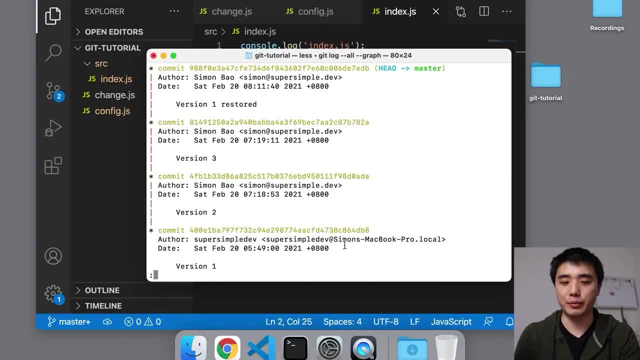 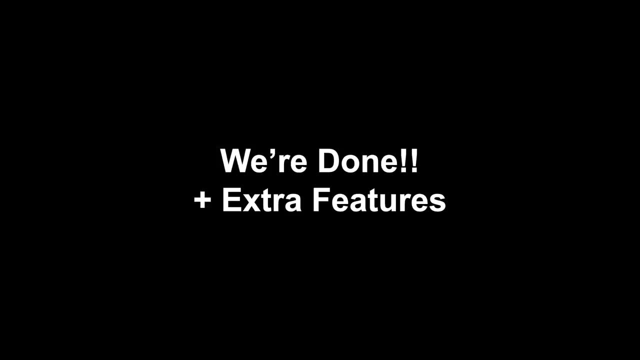 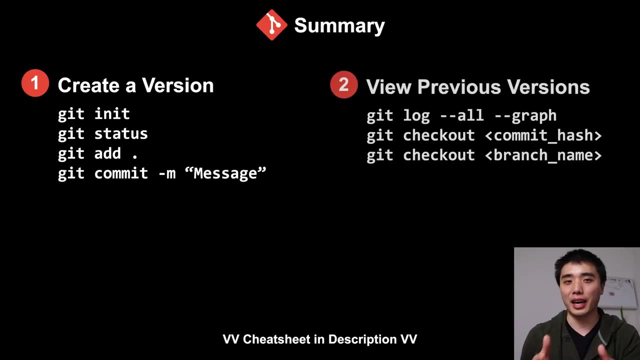 have any branching happening. And there you go. This is how we recreate the restore version feature from the Google Docs history. So I just want to say congratulations, because we just recreated the version history feature of Google Docs and Microsoft Word using git And now that we're done, comparing git with Google Docs version history. 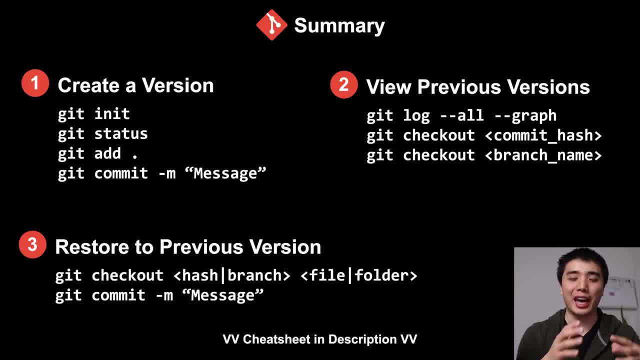 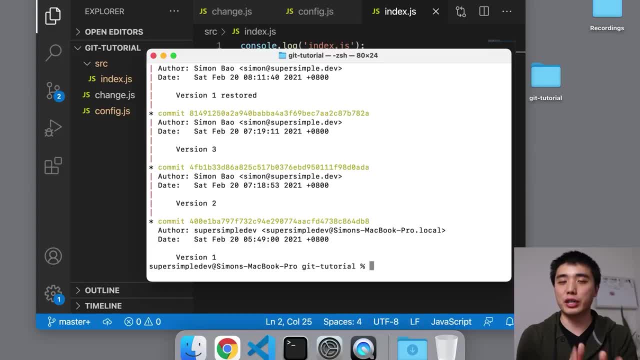 For the rest of this tutorial, I'm going to be using the words commit and commit history just to help you get familiar with the git terminology. So we finished the main project of recreating Google Docs version history using git, So now I'm going to show you some miscellaneous features of git that you'll find useful. 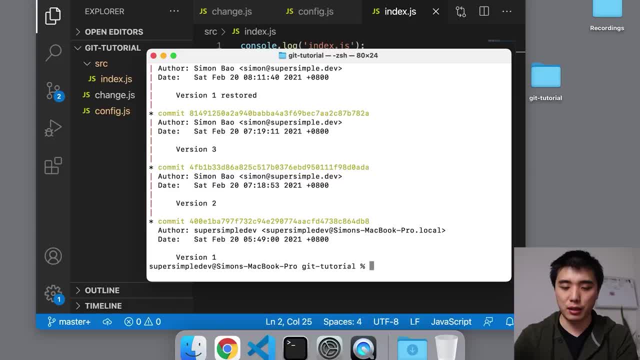 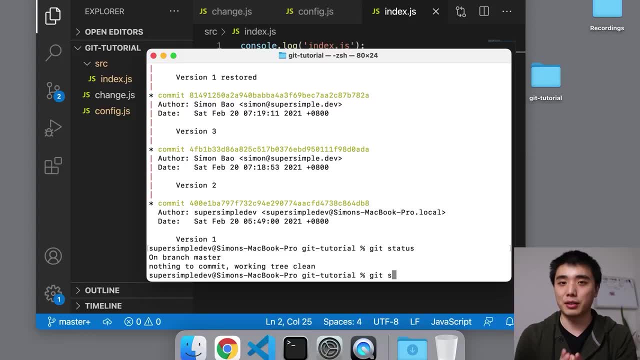 So the first feature I'm going to show you is like shortcuts. So instead of typing git status, instead I can type git s and it will do the same thing. So this is called aliases. Okay, So to type an alias, here's the git command: git config- dash, dash, global alias dot. 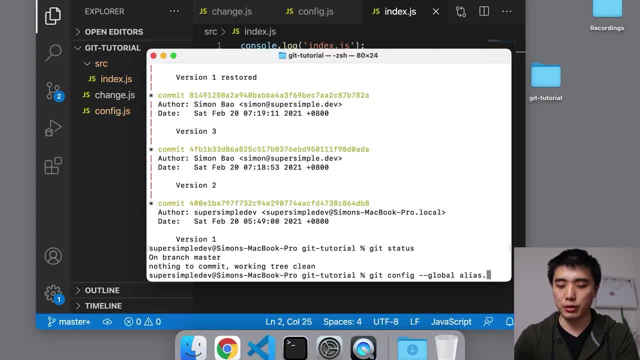 And then you're going to give the sort of shortcut that you want to use. So I'm going to use the shortcut s, and then I'm going to use the full command here to tell git what s should stand for. So s is going to stand for status. 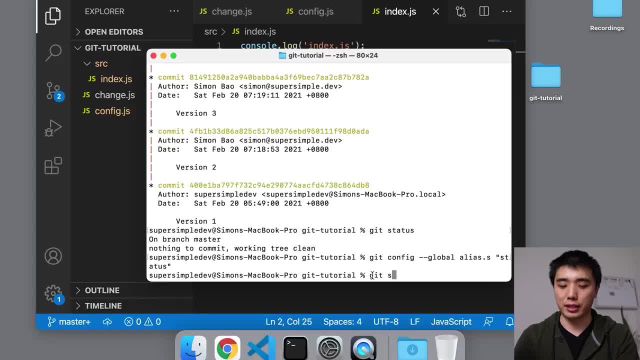 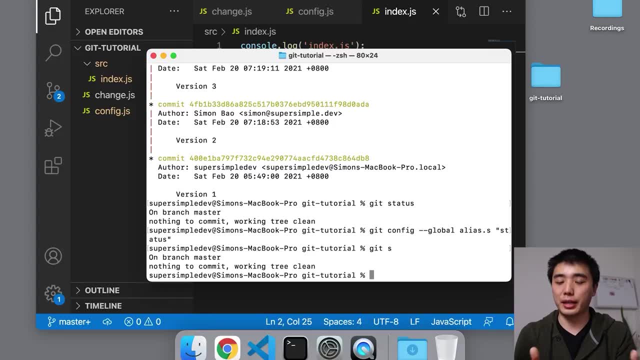 So next time when I type git s, git is actually going to run git status. So that's just a way to save you some typing and to make things go faster when you're working with git. So I'll share with you some of the aliases that I use. 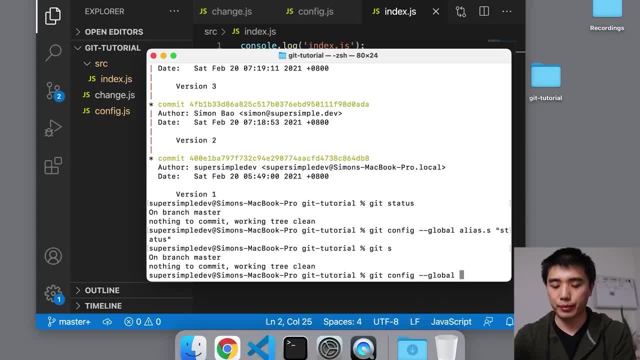 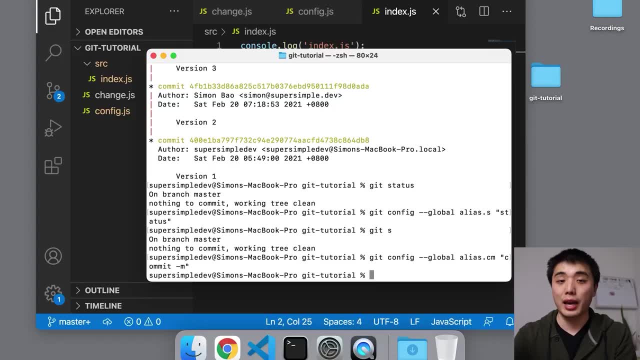 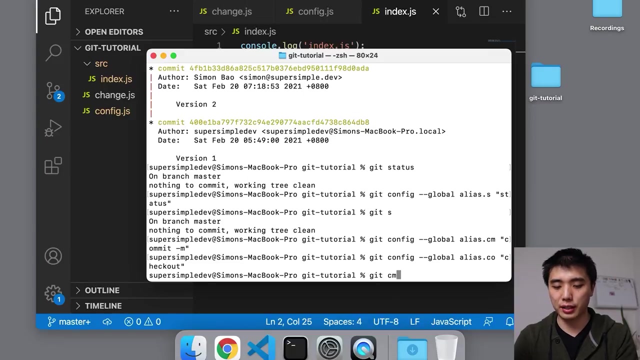 One of them is git config dash dash global alias dot cm, And I use this to represent commit dash m. And another one that's useful is git config dash dash global alias dot co, And I use that to stand for checkout. So now, instead of doing git commit dash m, I can just do git cm. 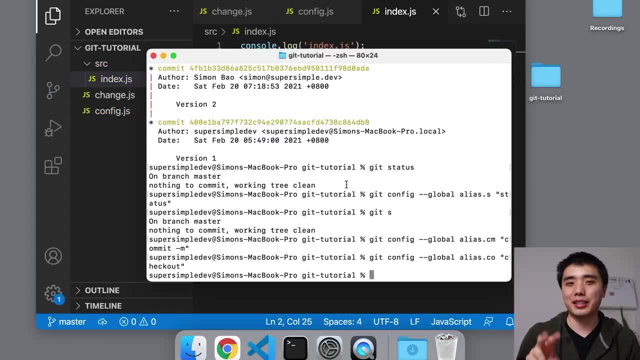 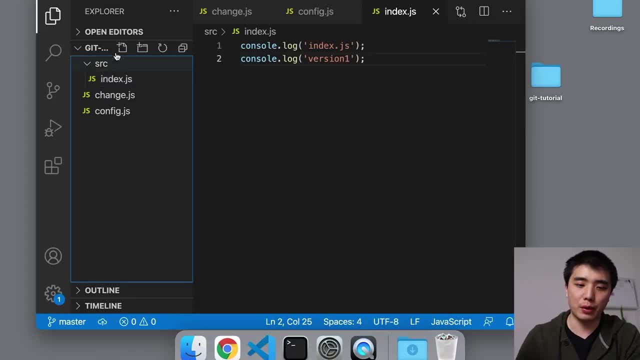 So I'm going to use the aliases that I use or create your own. So the second extra feature I want to show you is how to ignore certain files from being added to your version history. So this usually happens if you have a file like secret dot txt. 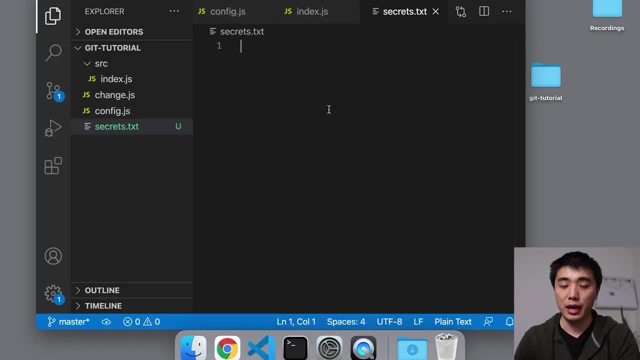 And inside this file there's a bunch of sensitive information, maybe some passwords, And you don't really want to put this in your version history because it will be saved forever. So what you can do is you can actually add a new file called dot git ignore. 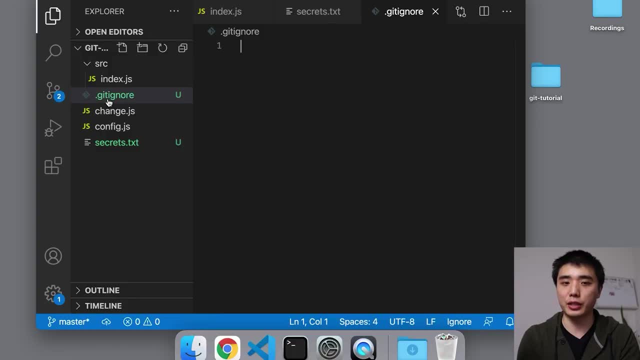 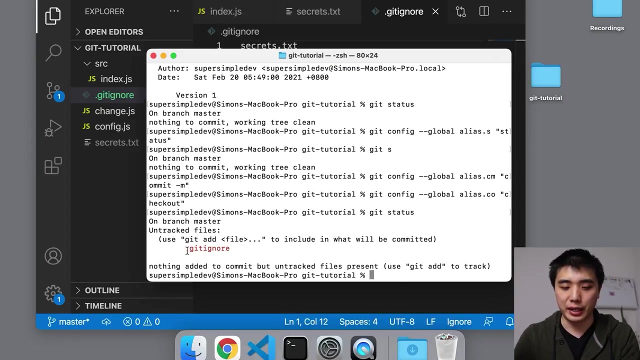 Okay, And this is going to tell git which files you want to ignore and not add into the version history. So we're going to put secrets dot txt into this file And then when we run git status, you can see that, because we have a dot, git ignore and 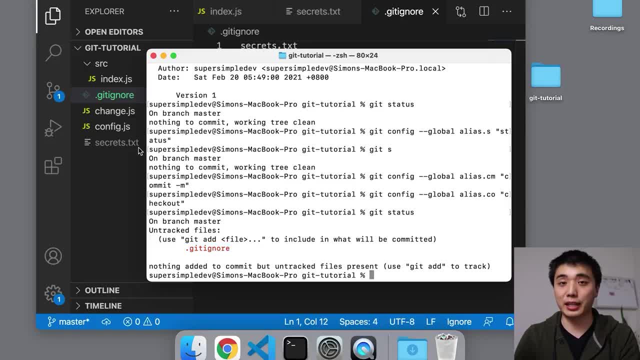 inside we specified we want to ignore this file. git is not tracking this file for changes. It's not going to add it to our version history. So this dot ignore file is actually a file that you should add. You can add it to your version history. 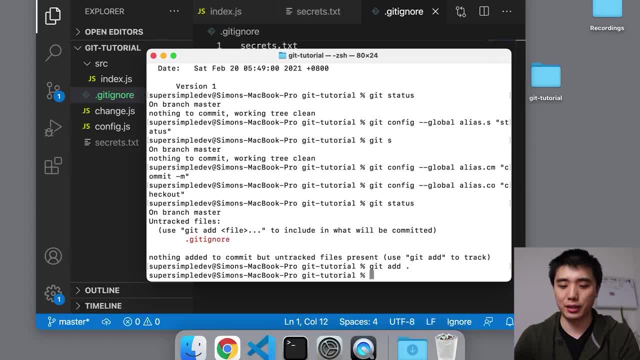 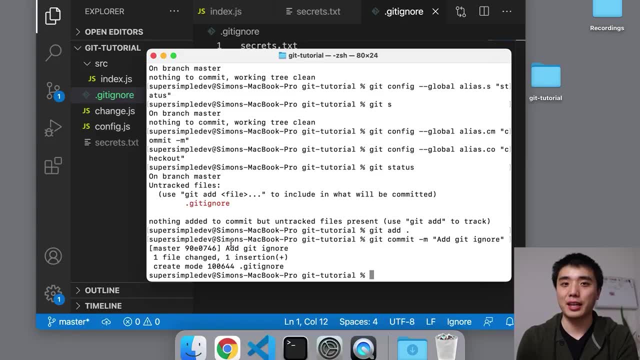 So we're going to add it right now: git add dot. git commit. dash m add git ignore. And that's it. That's how you prevent certain files from being tracked by git and being added to your version history. So the third and final extra feature I'm going to show you is how to completely remove git. 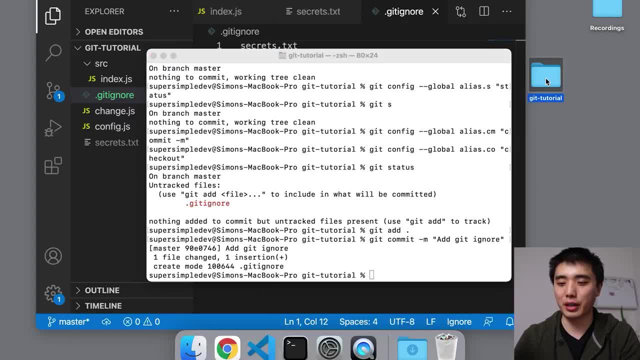 from your project. So first of all, let's create a copy of our project, because we'll need it later And we don't want to remove git right now, So we're going to paste that And I'm just going to call this. git tutorial dash two. 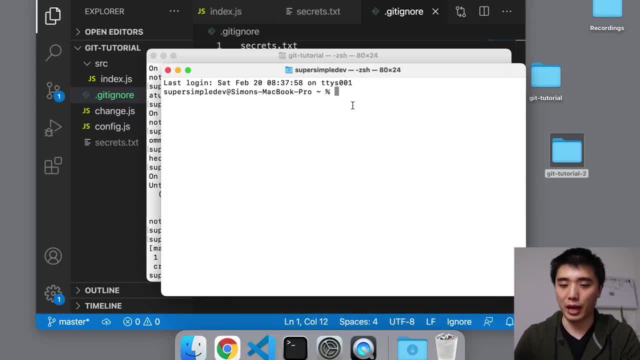 And now we're going to open a new command line and make sure that you change directory into this folder that contains a copy of all our code, tutorial two: And let's run git log again just to make sure that git is still in the copy of our folder. 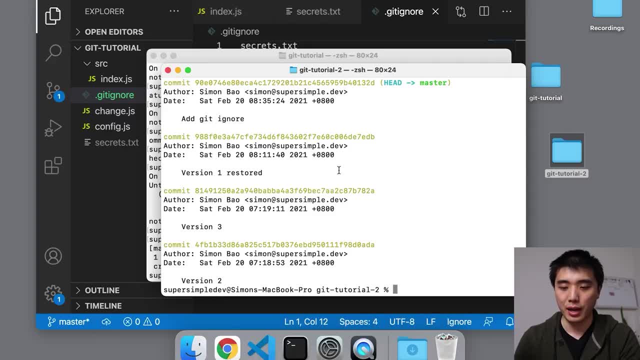 That's good. So to exit this, we're going to press Q for quit. Okay. And now to remove git from this project, all we have to do is give this command: rm, dash, rf, dot, git. So all of the data in git, including all of our commits or changes in our version history. 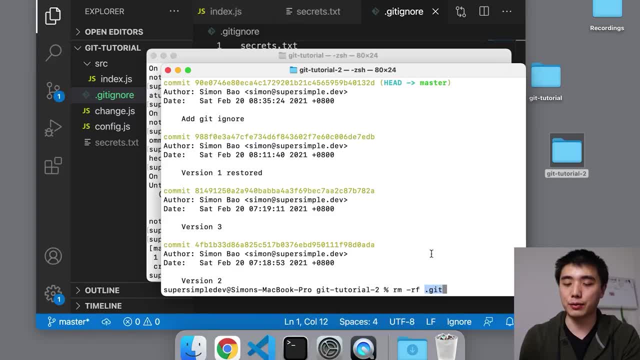 is saved in a folder called dot git, And if we just delete this folder, then we will remove git from our project, And this rm dash rf command basically removes this folder and everything inside this folder. So let's go ahead and run this command. 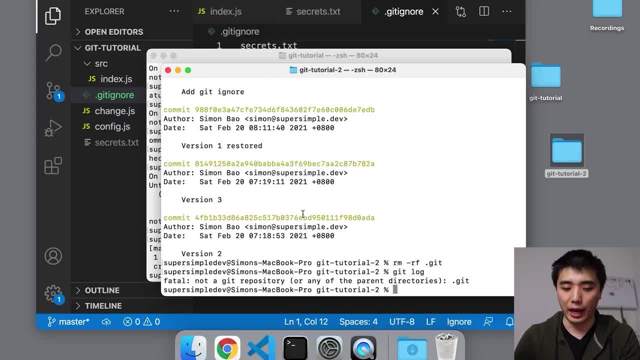 And now let's go ahead and run git log again, And you'll see that this is no longer a git repository. So a repository just means a folder that is being tracked by git, And that is how you remove git completely from your project.